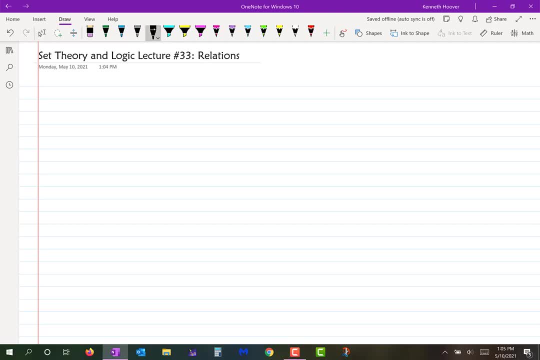 Okay, we're going to talk about relations today. Suppose you have a set A- Let's say this set has, we're just going to put some numbers in here. it's not important, particularly what they are. Okay. and another set B? Okay, let's do that. Let me make that six look better. Okay. now what if I say that? 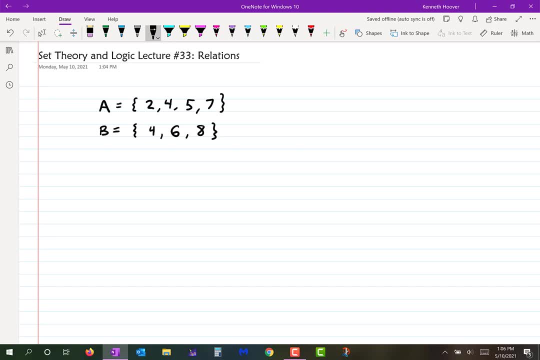 I'm going to write down how the numbers in A- which they might not even be numbers, they might be letters. so let me say elements, how the elements of A are related in a certain way To the elements of B, And let me draw this with an arrow diagram. Actually, I 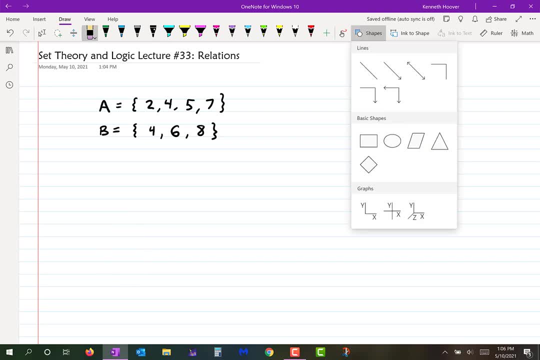 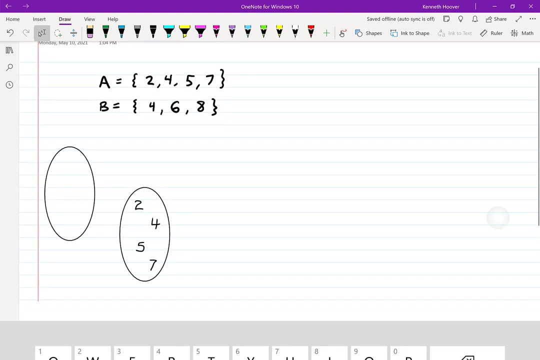 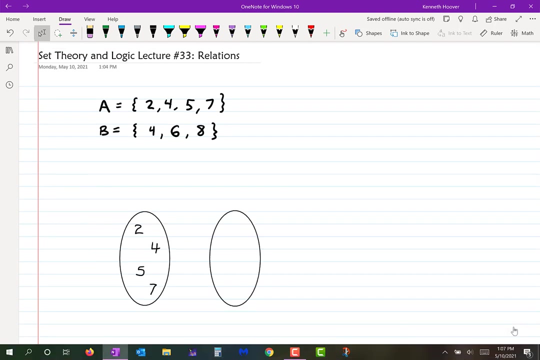 can do. I think let's see I can do a nice perfect shape like this. Okay, so let's put the numbers from A here, It doesn't matter Where I locate them. Okay, and then let's do something similar for B. Whoops, Ah, here we go. 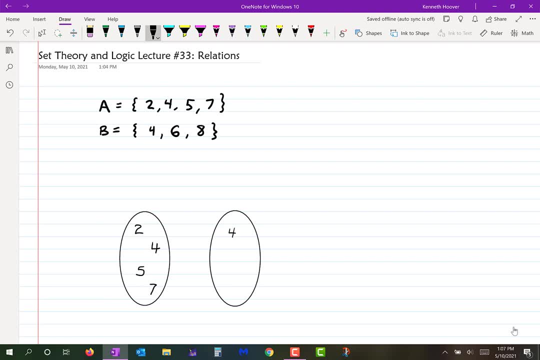 Okay, Alright. now what if I draw arrows like this: One arrow going from two to four? So two is related to four in some way- I'm not telling you yet what I have in my mind- And maybe two is also related to six, And maybe two is also related to eight. 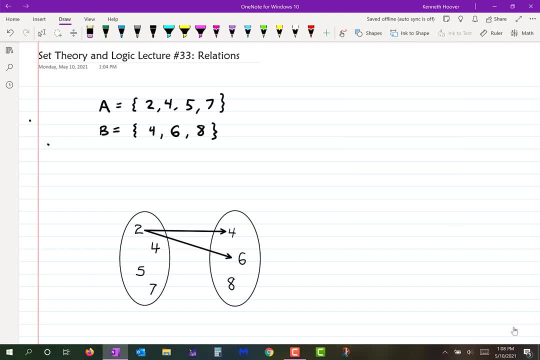 So two is related to all three of the numbers, Okay. And then let's do: four is related to six, Okay, So four is also related to all three numbers, But five is only related to six and eight. Okay, So five is only related to six and eight. 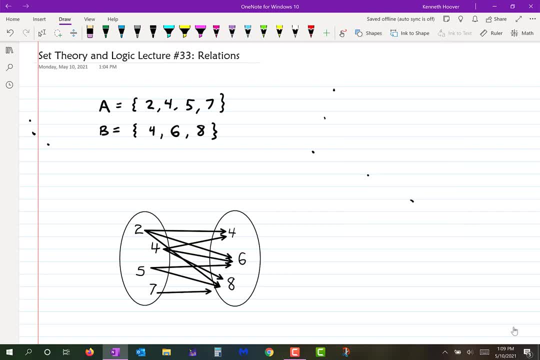 And seven is only related to eight. So there's a diagram showing how I want the numbers in A to be related to the numbers in B. Okay, So I'm not saying what the relation is here, I'm just telling you which numbers are related. 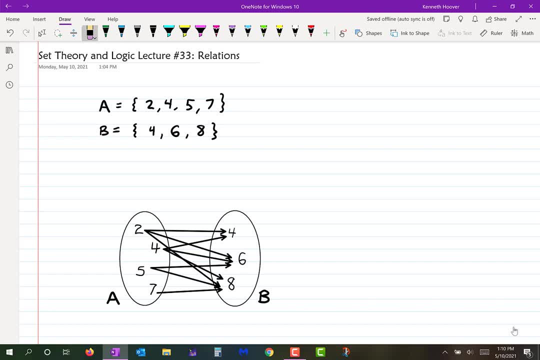 to others. Okay, Now this relation goes one direction. So I was about to say: I'm telling you which numbers are related to each other. Okay, Kind of like cousins, you know, and things like that. Okay, I stopped myself because that's not what I want to say. 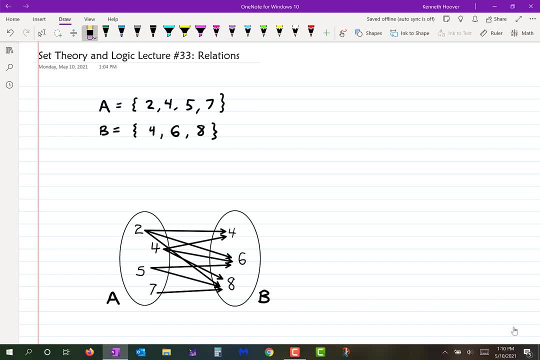 Because that's sort of a relationship. Okay, So that's sort of a relationship. It goes both directions. This one only goes one direction. Okay, Now I can do this. Let's call the relation R. Okay, Let's just call it R, And I like to draw an arrow like this: 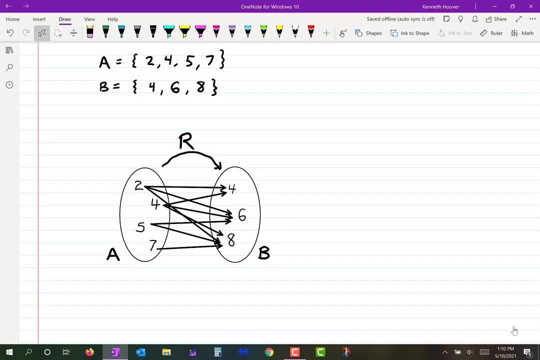 Okay, So that's saying this R is a, This is a relation from A to B. Okay, And this set A is called the domain of R. Okay, And this set A is called the domain of R. Okay, So I'm going to call this R, Okay. 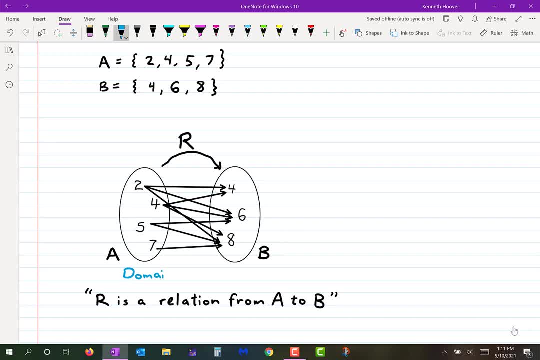 So let's call this R Okay. Let's call this R Okay, The R of the relation. Let's call this R Okay. And this set: B is called the co-domain, Not the range. In fact, I'm going to add another number to B. Let's add a one in there as well. 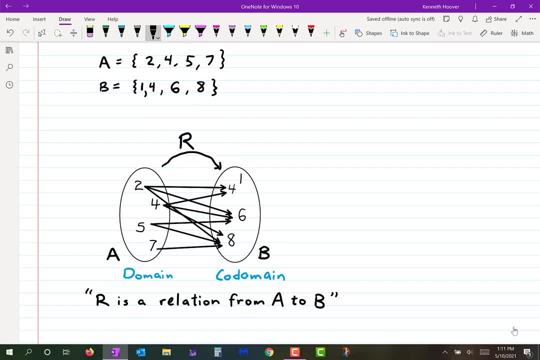 Okay, Let's do that, Okay, Okay, Let's find. So you see why B is not called the range? Because there are no elements of A that are related to the number 1 in B. That's why B is not called the range. 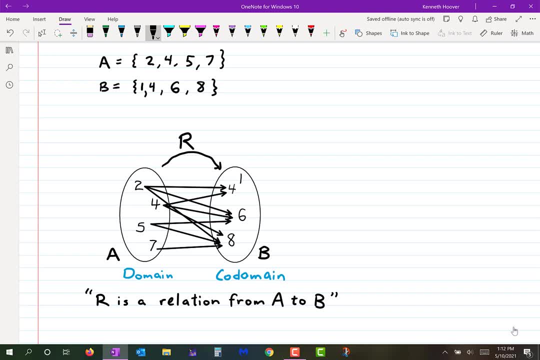 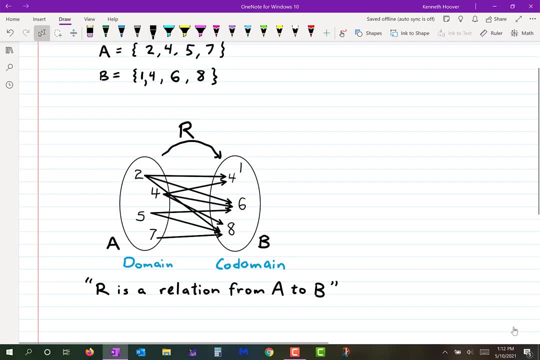 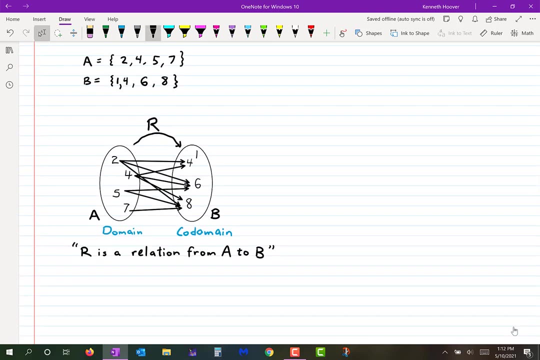 Okay, It's called the co-domain. Okay, Now I can write this. I can write: 2 is related to 4.. Okay, We write: 2 is related to 4.. We write: 2 is related to 4.. 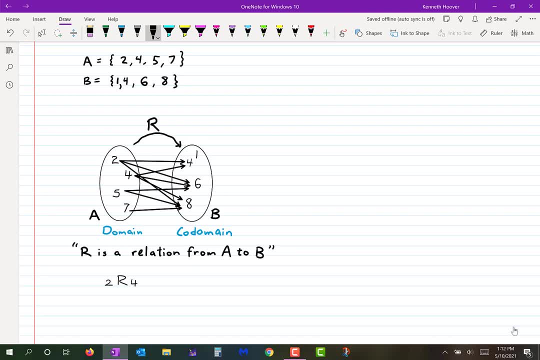 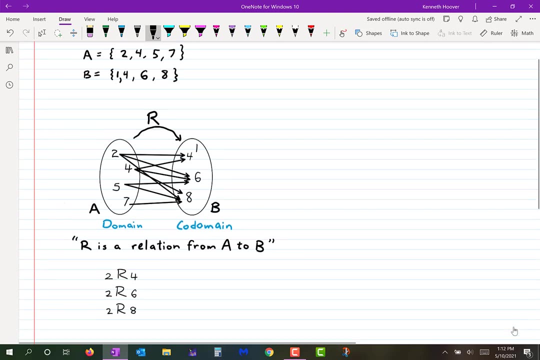 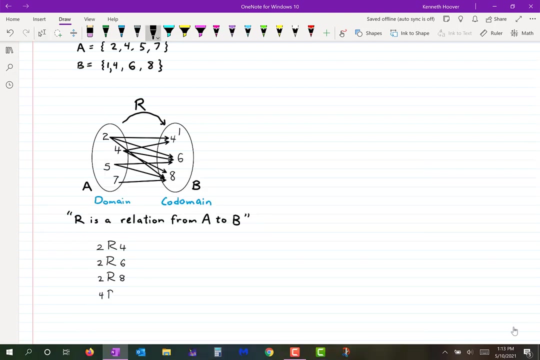 We write like that 2 is also related to 6. And 2 is related to 8.. I can say that 4 is related to 4.. 4 is related to 6. And 4 is related to 8.. 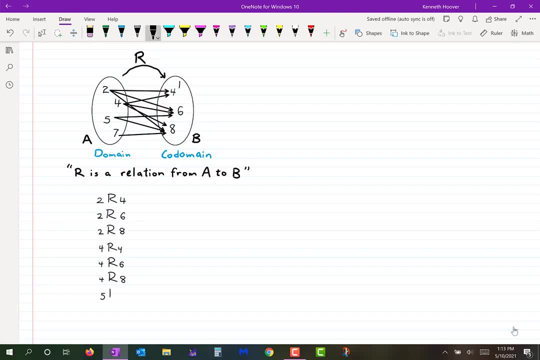 I can say that 5 is related to 6.. 5 is also related to 8. And I can say 7 is related to 8.. Okay, So here's one way of depicting a range. The relation is with this kind of a diagram. 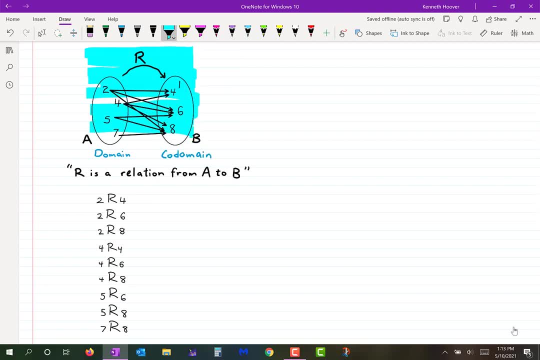 Certainly very visual, Really really gets the point across. But couple drawbacks: It takes up a lot of space, It tends to be time consuming to draw And one of the biggest drawbacks here is, you know, the strength of that diagram. 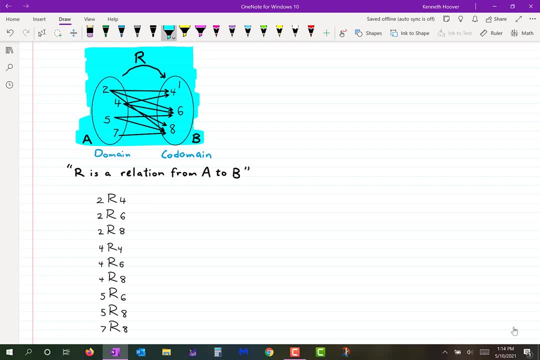 is that it's very visual, you can see the relationships. but that strength can also be a weakness. in this particular case, if there's too many arrows, then it just gets really hard for your eyes to follow the arrows, and i would say that this is almost bordering on that sort of a situation. it's not too crowded, but 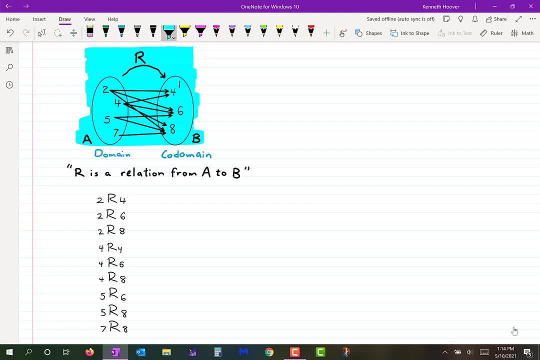 there are certain places in this diagram where the arrows overlap each other so much that it gets a little bit hard to follow them. okay, so arrow diagrams- very nice, very visual. tend to take a lot of room and time, though, to draw and can get way too crowded, in which case. 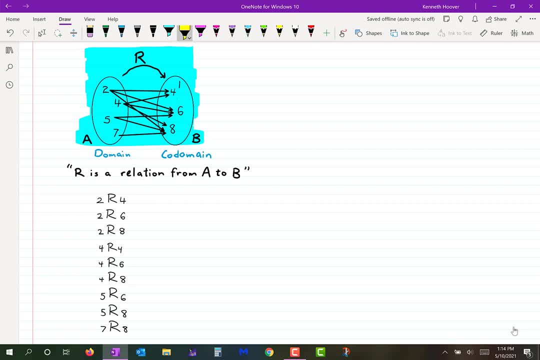 they just become almost useless. okay, so here's another way of representing the arrows, and the arrows are very similar to the arrows in the diagram. so here's another way of representing the arrows, and the arrows are very similar to the arrows in the diagram, representing a relation where you, you don't have to worry about overcrowding. 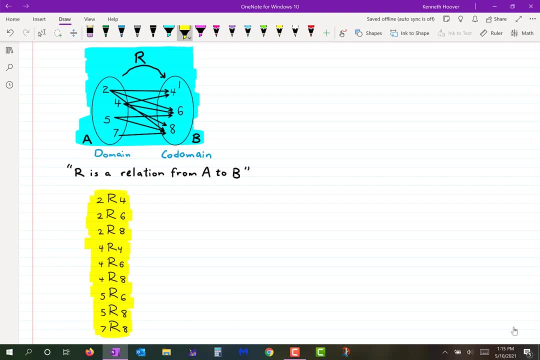 this is usually very quick to write down this. you lose the visual aspect, which is kind of a bummer. but it's quick and it's easy, okay, but it makes you ask the question. i wonder if there's an even more condensed way to write this. and there is, and and here's. another drawback too is that. 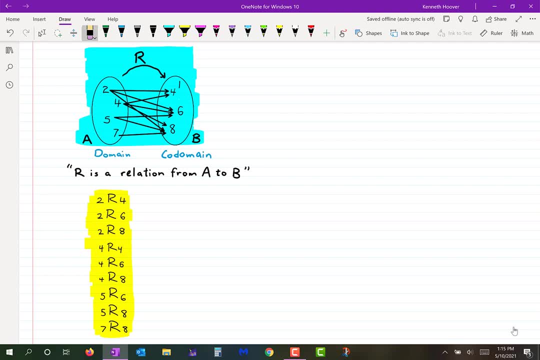 writing the relation the way i did there in yellow notice. it doesn't use any of the symbols that we've learned in this class from set theory. and you might say, well, yeah, but we, we've just learned a new symbol, which is that capital r. and that's true. but i do have the question: could i represent the? 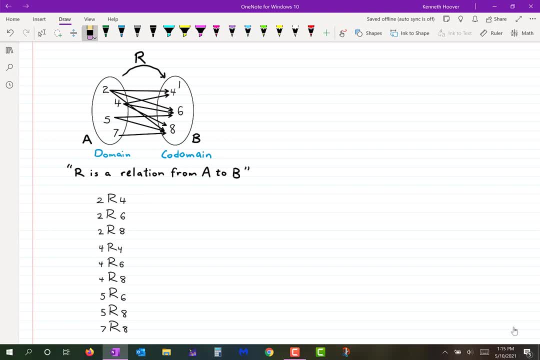 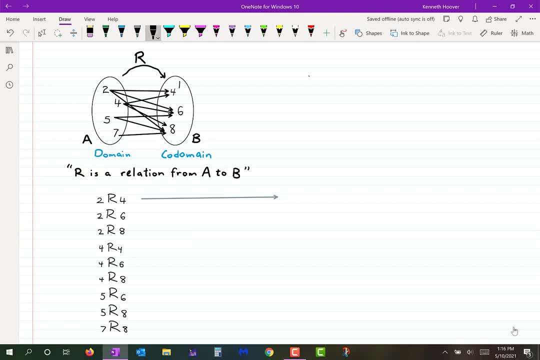 by just writing the ordered pair. oh, did i say two is related to r? i meant two is related to four. and i can rewrite that by just writing the ordered pair. oh, did i say two is related to r? i meant two is related to r. i meant two is related to r. i can represent that by just writing the. 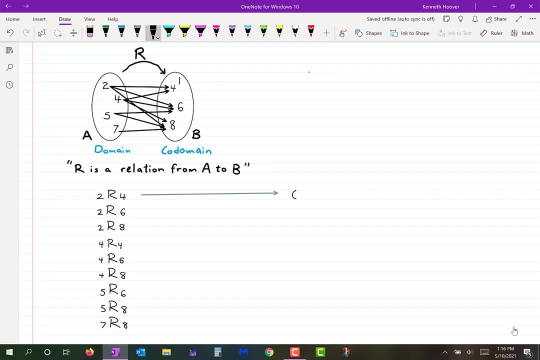 ordered pair two, comma four. and just asking you, when you see that, when you see the ordered pair two, comma four, say to yourself: two is related to four, next two and one- okay is two is related to six- can just be written as the ordered pair two, six and so on and so on. i'm gonna go ahead and 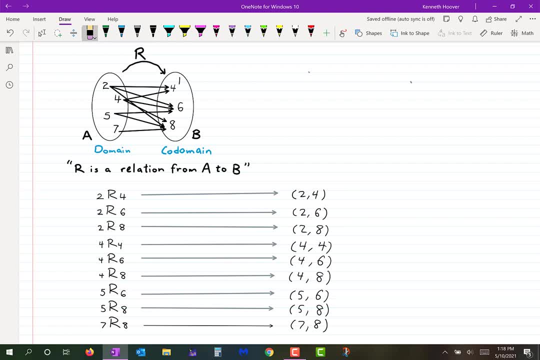 filling the rest. okay, there we go. so each of the relationships, and the relation R is the collection of all of those relationships, which means the relation R is the collection of all of these ordered pairs. what's another name for a collection? it's a set, right? a set is just a collection of things, right? 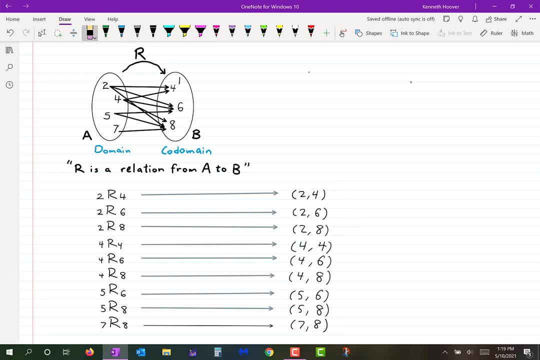 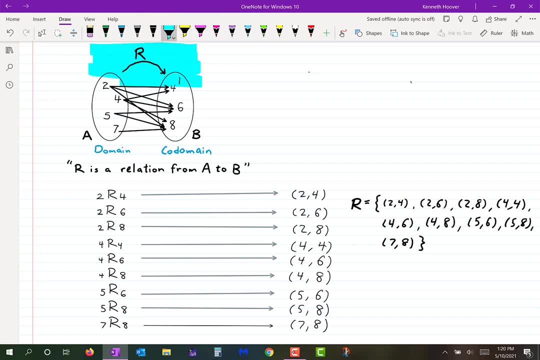 okay, there we go. so you see what I'm saying, let me just review okay. okay, there we go. so you see what I'm saying, let me just review okay. okay, there we go. so you see what I'm saying, let me just review. okay, this type of a thing here, that's. 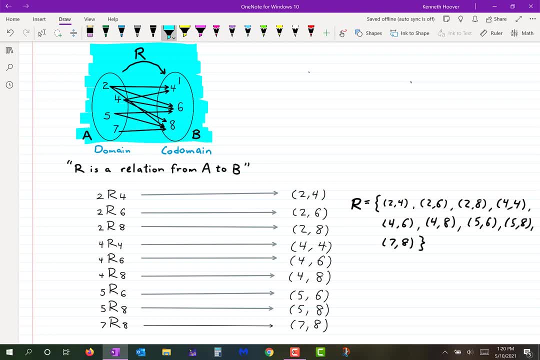 this type of a thing here. that's this type of a thing here. that's called a relation. a relation can also called a relation. a relation can also called a relation. a relation can also be represented like this: each be represented like this. each be represented like this. each individual relationship can be. 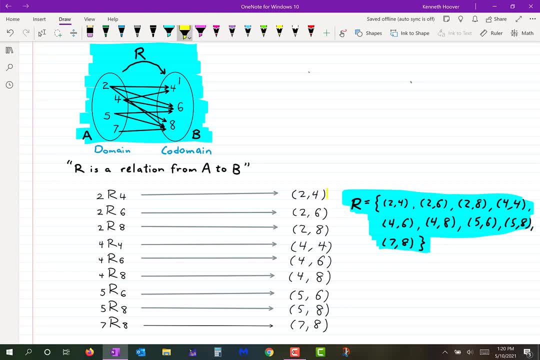 individual relationship can be. individual relationship can be represented as an ordered pair, represented as an ordered pair, represented as an ordered pair, or like this: okay, so in yellow, I've. or like this: okay, so in yellow I've. or like this: okay, so in yellow, I've shown you how to write individual. 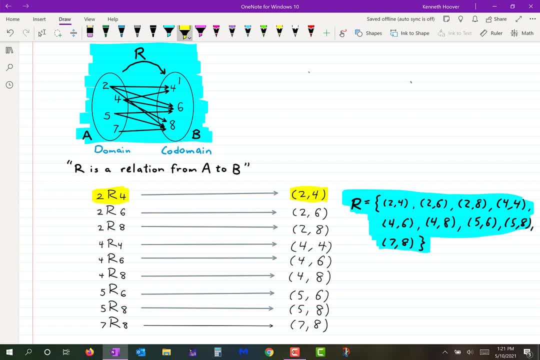 shown you how to write individual. shown you how to write individual relationships in blue. I've showed you relationships in blue. I've showed you relationships in blue. I've showed you how to write the entire relation- okay, how to write the entire relation- okay. how to write the entire relation- okay. got that. now I want you to notice. 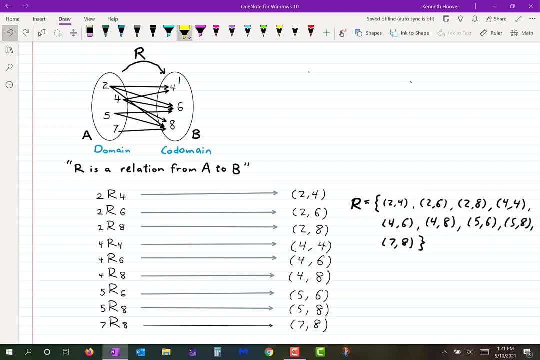 got that now. I want you to notice. got that now. I want you to notice something really important. if I'm something really important, if I'm something really important, if I'm right. the relation this way, what is that right? the relation this way- what is that right? the relation this way- what is that? that's just a set of ordered pairs, right? 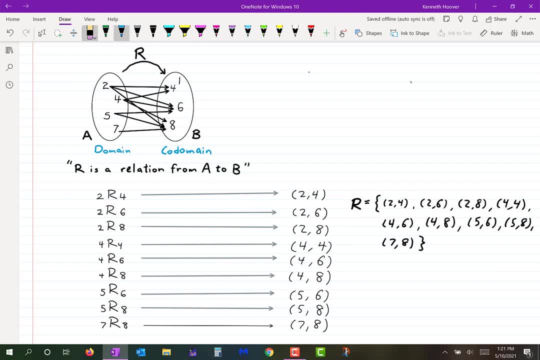 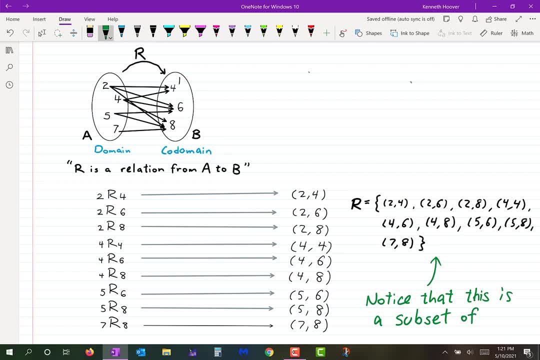 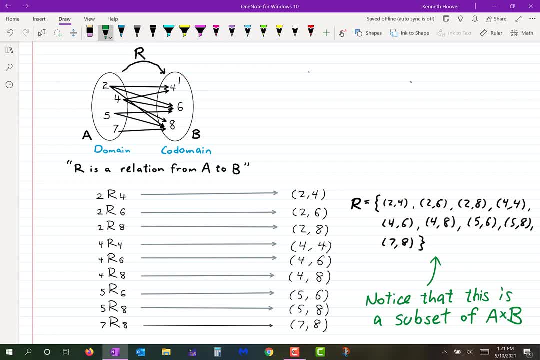 this is really important for you to this is really important for you to understand every relation from a set a. to understand every relation from a set a, to understand every relation from a set a to a set B can be represented by a subset. a set B can be represented by a subset. 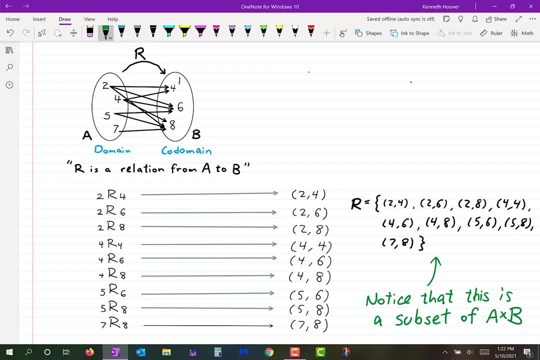 a set B can be represented by a subset of a cross B. and let me say the same of a cross B, and let me say the same of a cross B, and let me say the same thing in the other direction, every thing in the other direction, every. 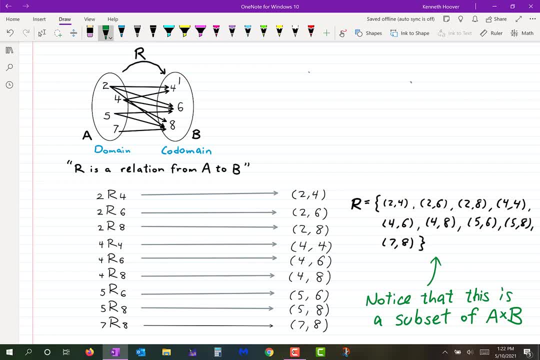 thing in the other direction. every subset of a cross B represents a subset of a cross B represents a subset of a cross B represents a relation from a to B. I'm going to put relation from a to B. I'm going to put relation from a to B. I'm going to put that here in writing. every relation from 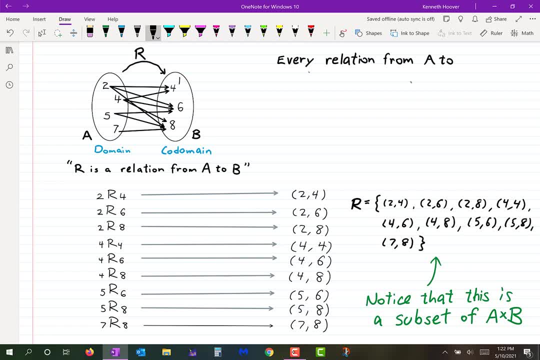 that here in writing. every relation from that here in writing. every relation from a to B can be represented by a a to B can be represented by a cross B as a subset of a cross B. also, every a to B can be represented by a cross B as a subset of a cross B. also, every 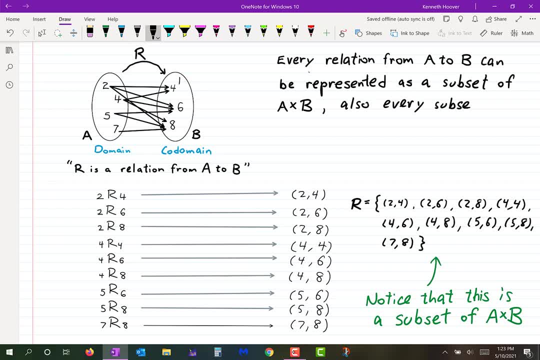 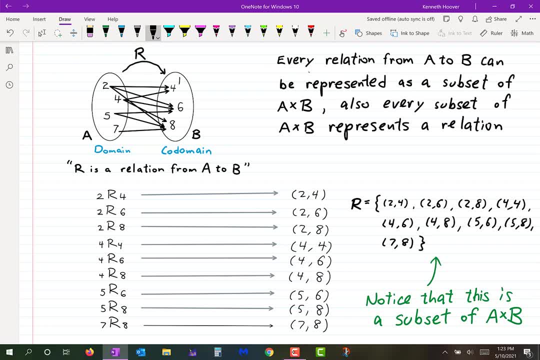 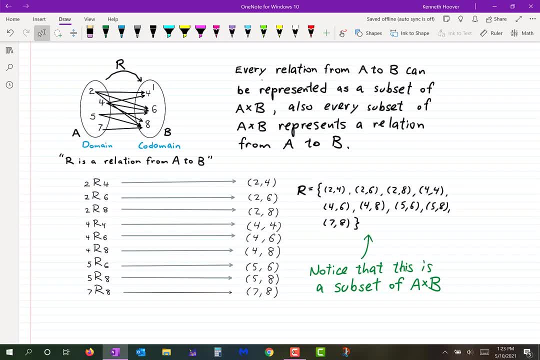 that relation that I've showed you right here is actually a relation that you already know. some relations represent things that you know already and some don't. okay, look at that and see if you can tell. what I'm trying to say is this: when I drew those arrows in that diagram up there, I was 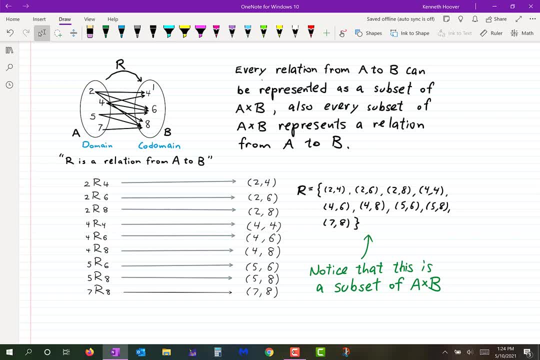 following a certain rule in my head. that's what I'm trying to say. okay, I was following a certain rule in my head to determine where I should draw the arrows. if you were to look at that, pretend this is like a game, a riddle. look at that diagram, see if you can figure out what rule I was. 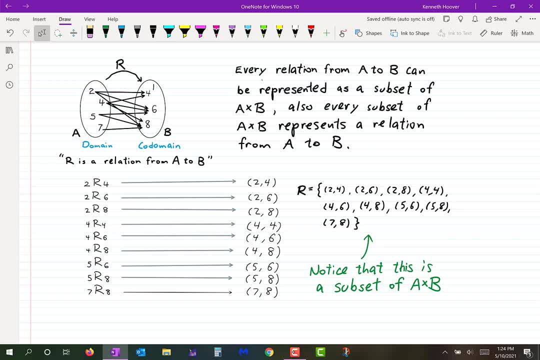 using. can you figure it out? okay, I'm going to give away the answer: positive, if you want to wait, if you don't want a spoiler, okay, the rule I was following is the rule is less than or equal to. okay, do you see that two is less than or equal to four, twos less than or equal to? 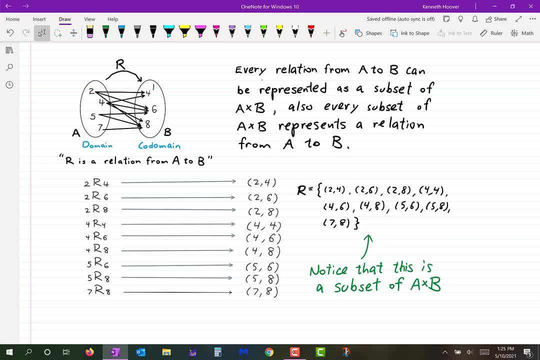 six. twos less than or equal to eight. two is not less than or equal to one. four is less than or equal to four. four is less than or equal to six and four is less than or equal to eight, but four is not less than or equal to one. five is less than. 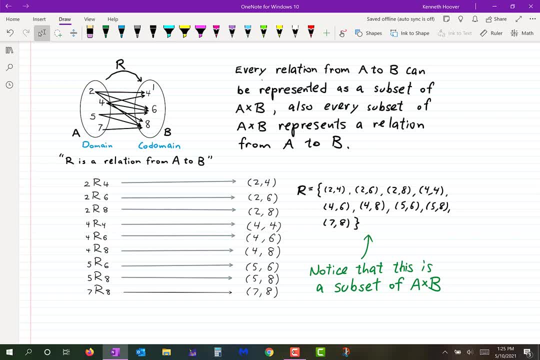 or equal to six and five is less than or equal to eight, and, but it is not less than or equal to one, and it's not less than or equal to four. and seven is less than or equal to eight, but seven is not less than or equal to one, it's not less than or equal to four and it's not less than or equal to. 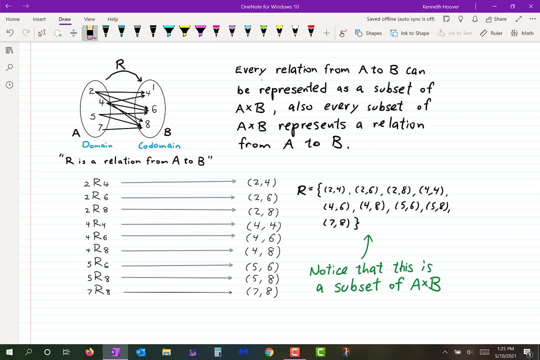 six. so that relation that I drew is in fact the relation that I drew is in fact the relation less than or equal to. okay, and in fact in this column here, since there's a symbol for less than or equal to, I could have used that symbol. okay, so that's. 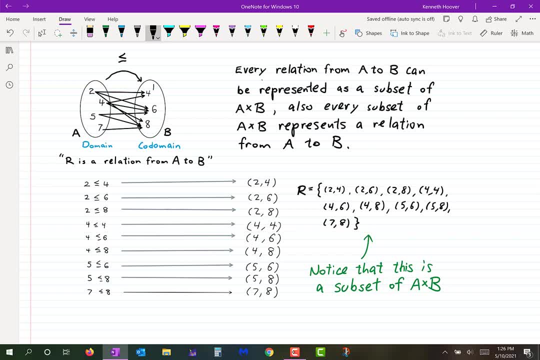 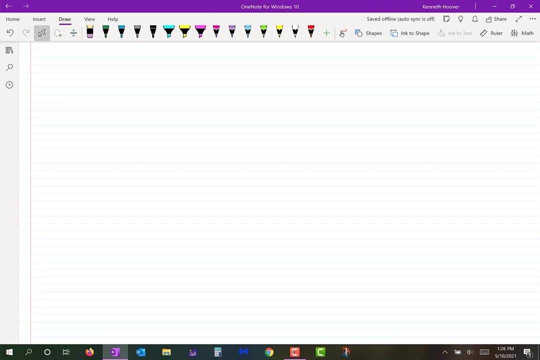 what a relation is, what a relation is now. you can have a relation that goes now. you can have a relation that goes now. you can have a relation that goes from a set to itself- okay. a relation from a set to itself: okay. a relation from a set to itself- okay. a relation from, let's say, from a set a to a. I'm 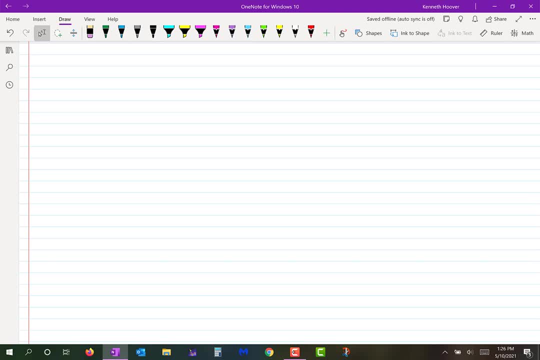 from, let's say, from a set a to a. I'm from, let's say, from a set a to a. I'm going to do a different one this time, going to do a different one this time, going to do a different one this time. here, let's say: a is the set this time. 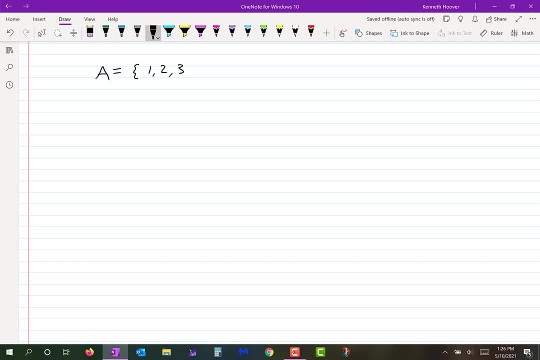 here let's say a is the set this time. here let's say a is the set this time. let's say 1, 2, 3 & 4. okay, and I'm gonna. let's say 1, 2, 3 & 4. okay, and I'm gonna. 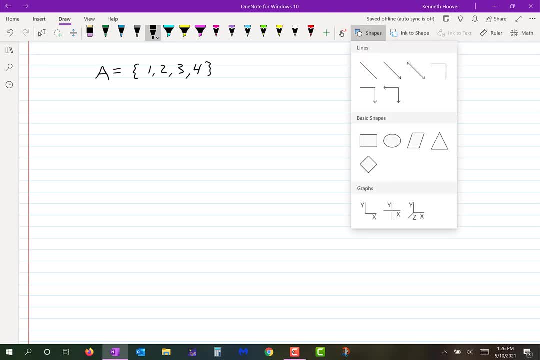 let's say 1, 2, 3 & 4. okay, and I'm gonna draw a relation from a to a. all right, draw a relation from a to a, all right. So 1,, 2, 3, 4, 1,, 2, 3, 4.. Let's put the arrows in there. Okay, and I'm gonna do the relation. 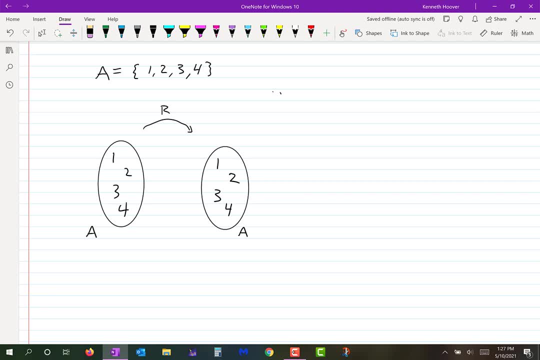 like this. Let me think for a second here. Okay, I don't want to make it too crazy, Let's just do. let's do this. 1 is related to 3.. Ah, and it's also related to itself. I would like to do that. 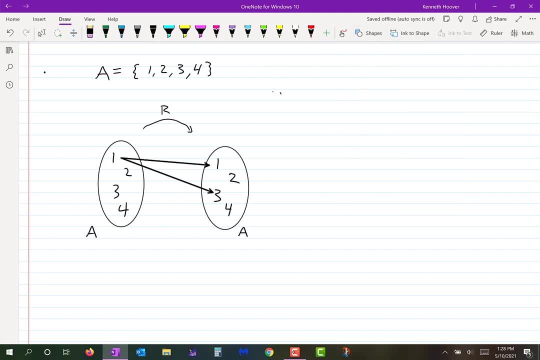 2 is related to itself, and also for 3.. I want to make related to 1 and itself- Okay. and 4 I would like to make related to 2 and itself- Okay. so there's a few things I can write. 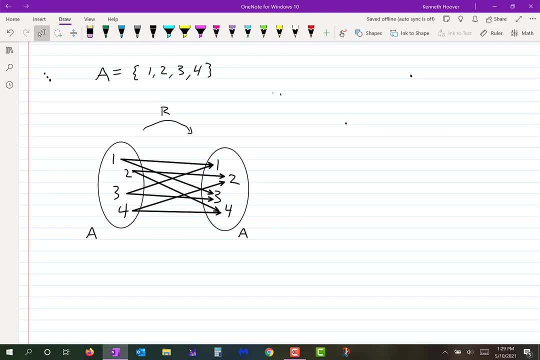 I can write: 1 is related to 1.. Let me make this smaller. I can write: 1 is related to 1 and 1 is related to 3 and 2 is related to 2 and 2 is related to 4 and 3 is related to 1 and 3 is related to 3.. 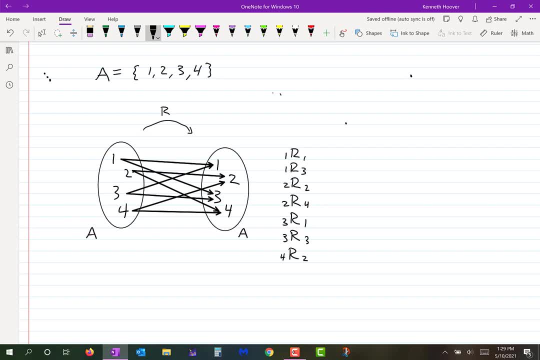 And 4 is related to 2 and 4 is related to 4.. Or I can write: the relation equals the set of ordered pairs: 1, 1,, 1, 3,, 2, 2,, 2, 4, 3, 1,. 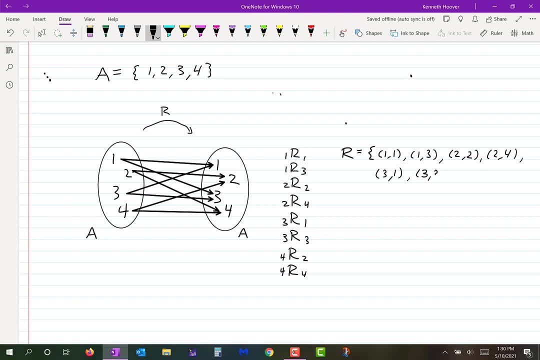 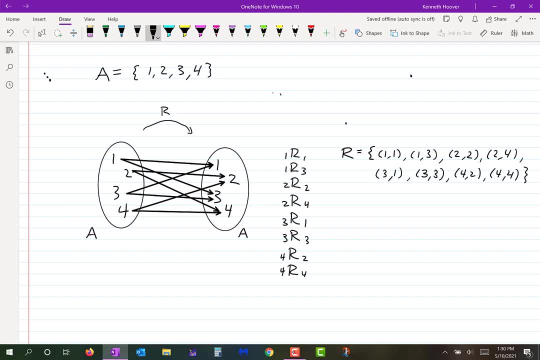 I could literally just put in random arrows. Okay, However, I didn't. I actually did follow a rule this time, just like last time. can you figure out the rule? see if you can figure it out. it's not as simple as the last one, though. okay, the rule is this: a number is. 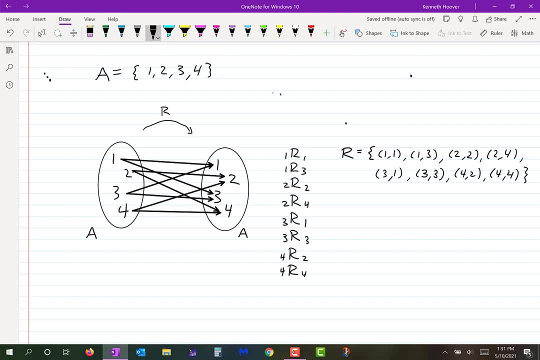 related. let me say that, say this way: a number in the domain is related to a number in the co-domain if, and only if, the number in the co-domain has the same parity. okay, so I can write a couple of things. I can say: X is related to Y if 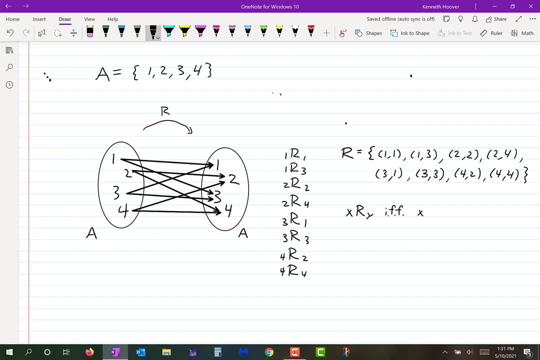 and only if X and Y have the same parity. okay, that's the relation that I drew in that diagram, or another way of writing, that is to say, X comma Y is an element of the relation if, and only if and only if, X and Y have the same parity. 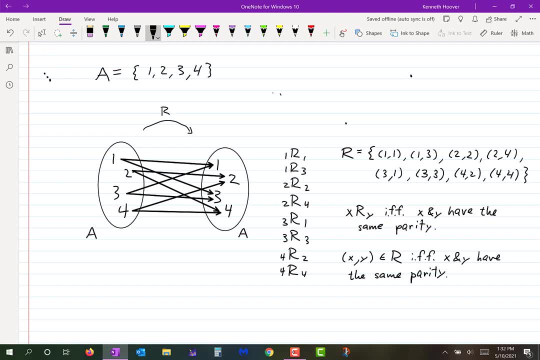 okay, now notice that the domain and the co-domain are the same in this particular case. so I would say, for example, if I have the same number of images, erosions, and I'm sorry. on the other hand, if I have some aberrations or directly different content or�s that are linked to each other in this particular policy. 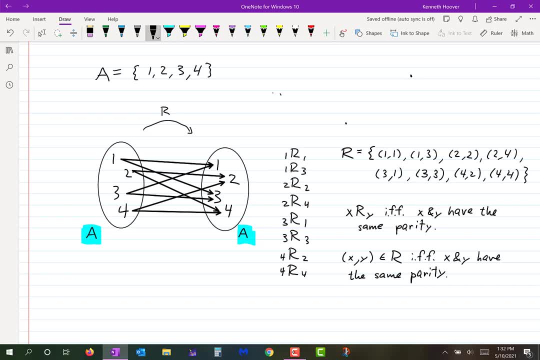 and this policy must be so. you can. you can see inside here, in the code located inside x, y are нами. first of all, this would be correct to say: R is a relation from A to A. That is mathematically correct. There's a correct use of language. But there's something else I could say. that's: 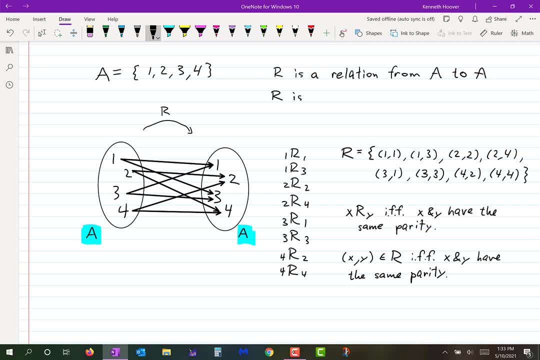 slightly shorter is. I can say R is a relation on A. Okay, So on A is the same thing as saying from A to A, Just using the mindset that if the domain and codomain are the same, then why say that name twice? Okay. 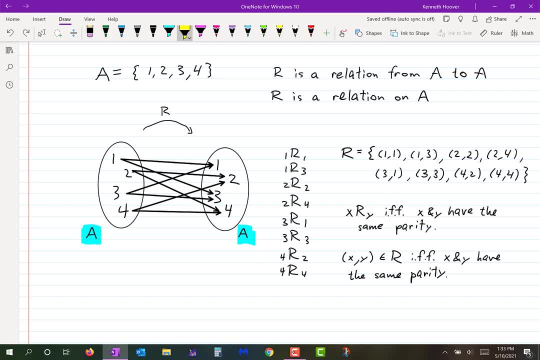 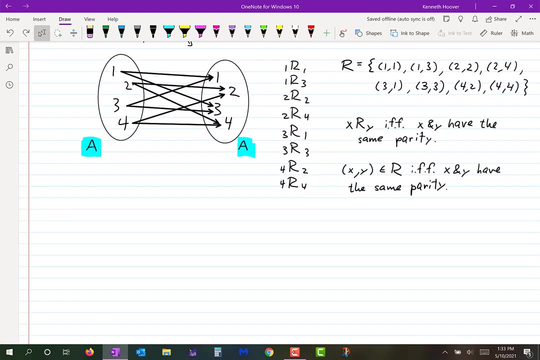 Now you might also ask this question: Since the domain and the codomain are the same, then why draw them twice in the diagram? And that's a good point, And you don't have to draw them twice. You could have done this. Or I could say: I could have done this, I could. 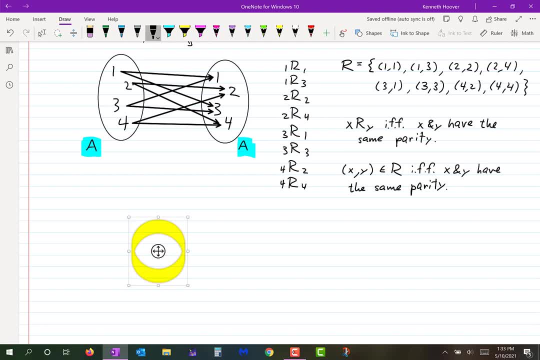 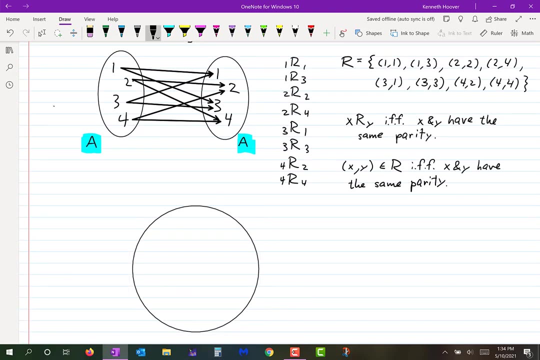 have just drawn A once. Whoops, I'll make it a little bit bigger here. Okay, so it's not crowded. I could have done this And I could have said: one is related to itself And it's also related to three. 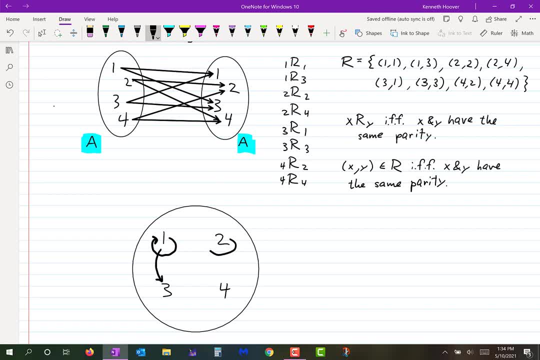 2 is related to itself and it's also related to 4. 3 is related to itself and it's also related to 1. 4 is related to itself and it's also related to 2. I could have drawn the diagram that way. okay, it's just a matter of how you'd. 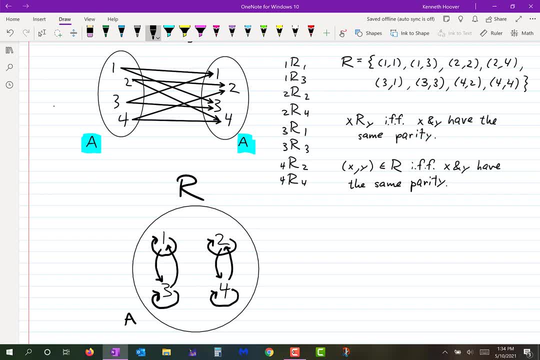 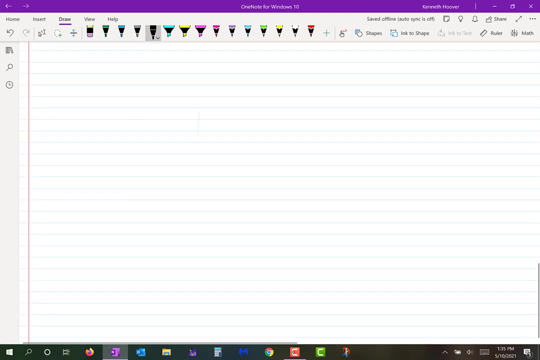 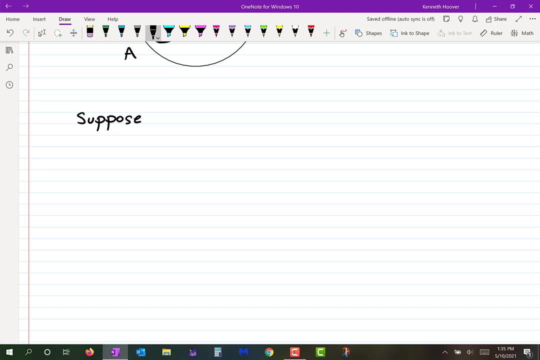 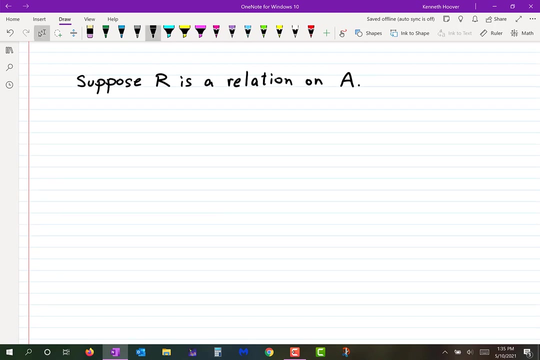 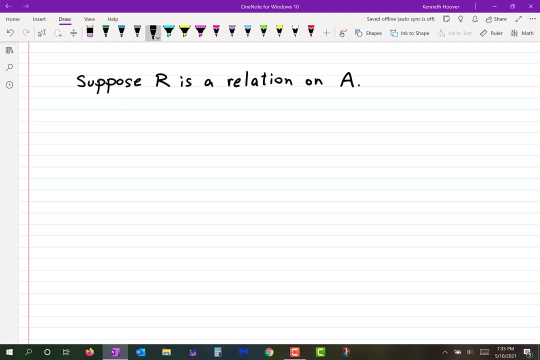 on a okay, there are some adjectives on a okay, there are some adjectives that are might earn or it might not. that are might earn or it might not. that are might earn or it might not. there's three in particular okay, so R is. there's three in particular okay, so R is. 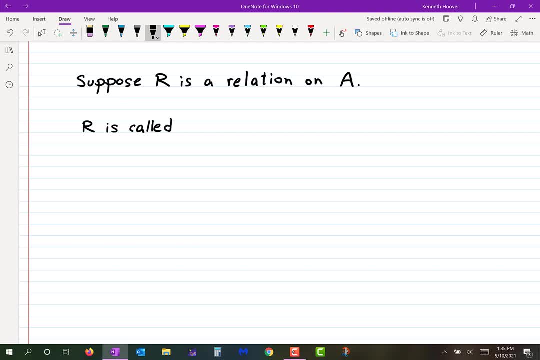 there's three in particular. okay, so R is called reflexive, called reflexive, called reflexive. if X is related to itself, for every X in a. if X is related to itself, for every X in a. if X is related to itself, for every X in a. actually, I'm gonna, I'm gonna word it. 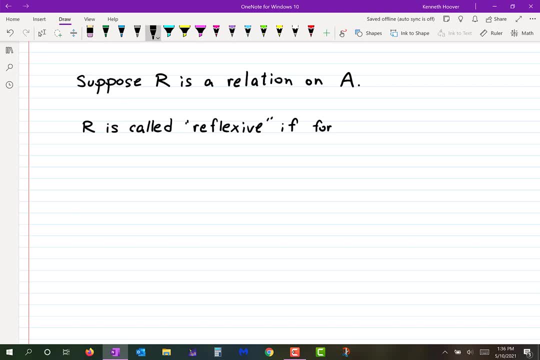 actually I'm gonna, I'm gonna word it. actually I'm gonna. I'm gonna word it like this: if for every X in a, we have a like this, if for every X in a, we have a like this, if for every X in a we have a, X is related to itself. another way of 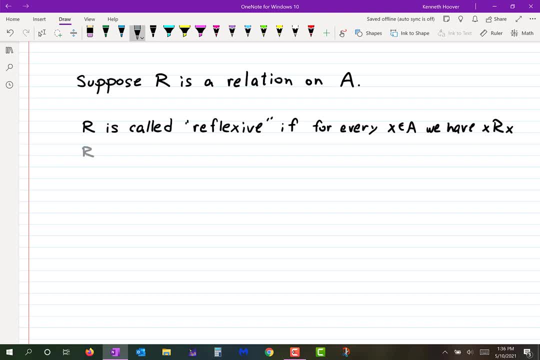 X is related to itself. another way of X is related to itself. another way of saying that is to say R is called saying. that is to say R is called saying. that is to say R is called reflexive if the ordered pair X comma X reflexive. if the ordered pair X comma X. 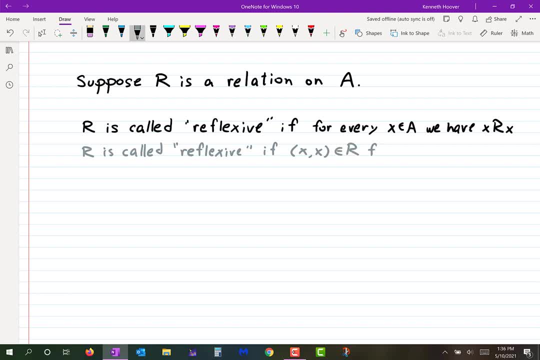 reflexive if the ordered pair X, comma X is an element of R, is an element of R, is an element of R for every X in a, so that's reflexivity. okay, all for every X in a, so that's reflexivity. okay, all for every X in a. so that's reflexivity. okay, all right, here's another adjective that a. 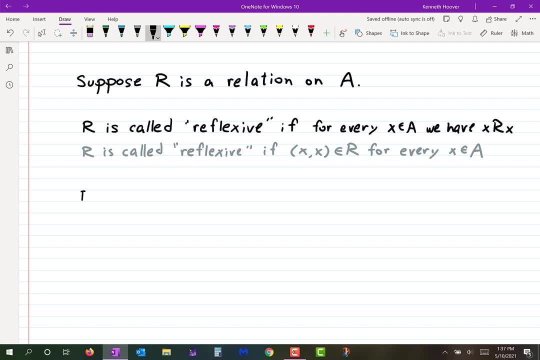 right. here's another adjective that a right. here's another adjective- that a relation might have R is called symmetric relation. might have R is called symmetric relation. might have R is called symmetric, symmetric, symmetric, if X being related to Y implies that Y is, X being related to Y implies that Y is. 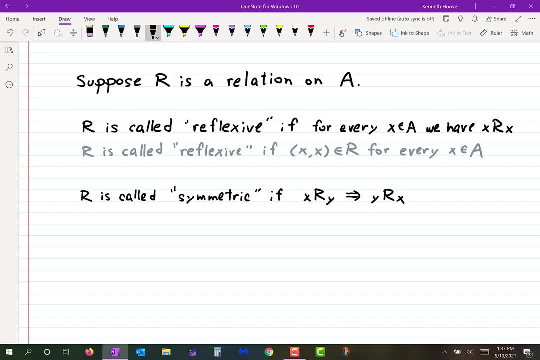 X being related to Y implies that Y is also related to X, also related to X, also related to X. remember, when we say a mathematical, remember when we say a mathematical, remember when we say a mathematical relation, it does not necessarily work in relation, it does not necessarily work in. 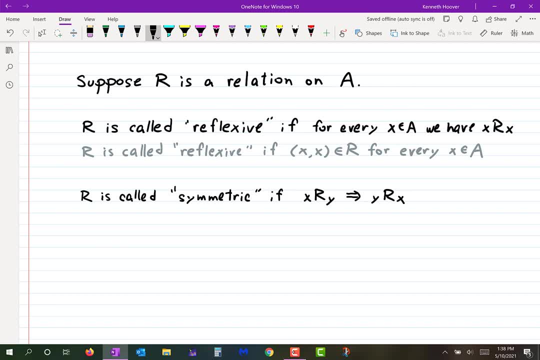 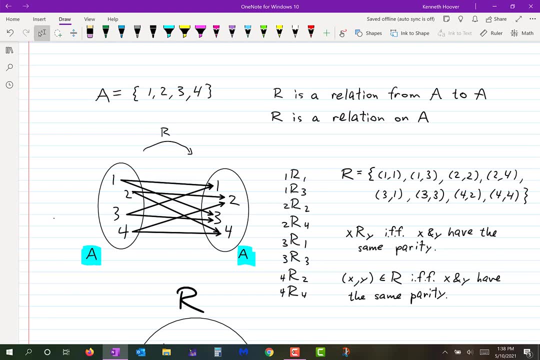 relation. it does not necessarily work in both directions. remember this one up both directions. remember this one up both directions. remember this one up here. let's look at the first example here. let's look at the first example here. let's look at the first example. sorry, that's not the first example here's. 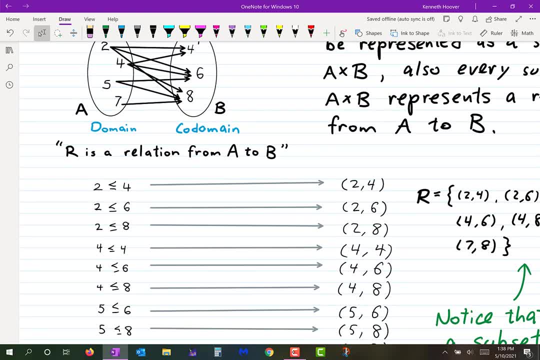 sorry, that's not the first example here's. sorry, that's not the first example. here's the first example, the first example. so notice that 2 is related to 4, but 4 was not related to 2. okay, so this is a relation, that is, you could say it's unidirectional instead of bi-directional. 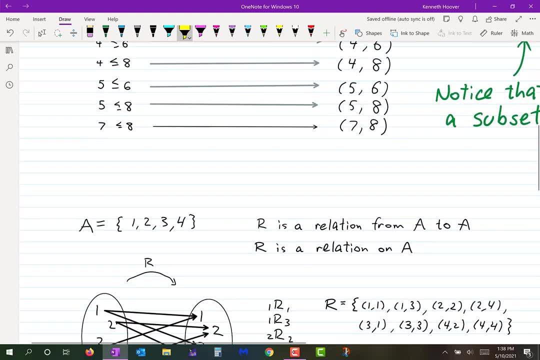 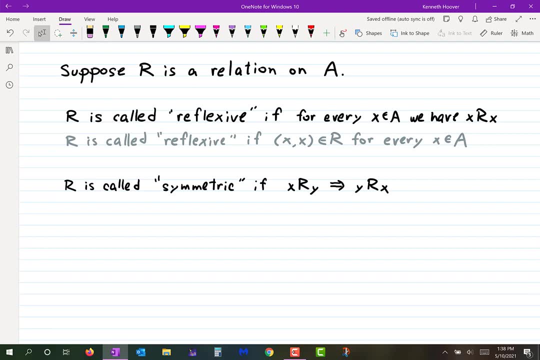 okay. but what's better is to use the correct terminology and say it is not symmetric. okay if X being related to Y automatically means that Y is also related to X. in that case you would call it a symmetric relation. okay, or another way to write, that is to say R is called. 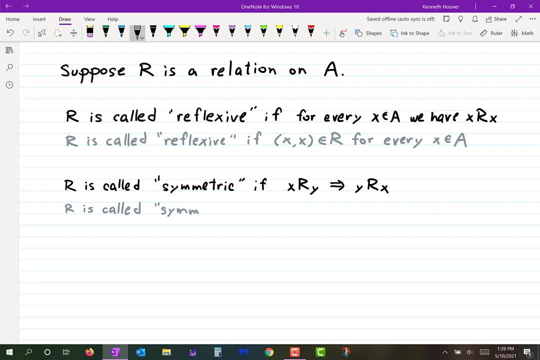 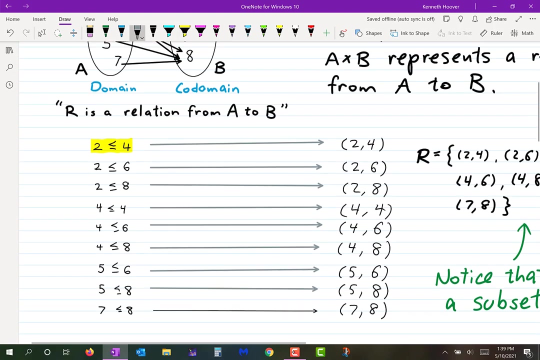 symmetric if we let's write it like this: if for every X, Y that is in R, we have Y, X is also in R. so again, I'm going to go back to that first relation and show you that it's not symmetric, because I'm going to use the same example, because 2, 4 is in the 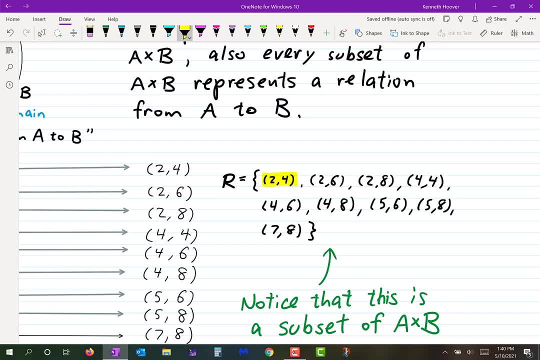 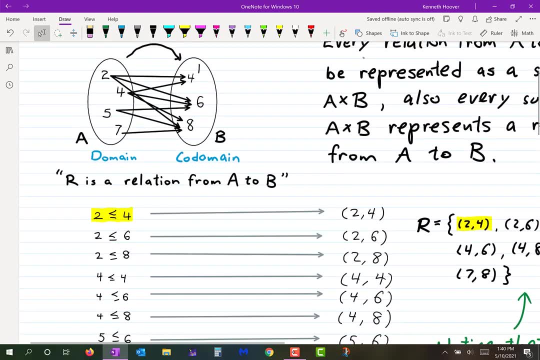 relation. but if you look there, you see that 4: 2 is not, actually, to be honest with you, even there's, even so, that's why this is not symmetric. okay, yes, but I also just realized something, and then I'm going to go back to that first relation. 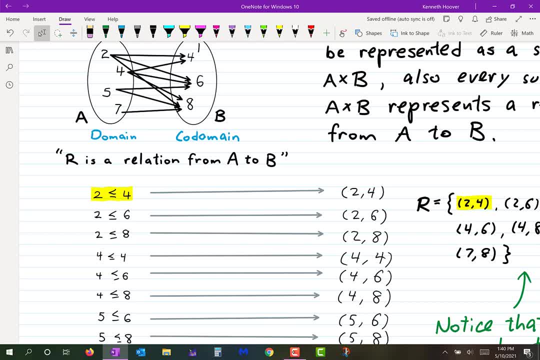 this does not ruin the examples that I've said so far, that I just happened to notice this- that this could not have possibly been symmetric anyways, because the domain and the co-domain aren't the same set. this is not a relation on a set, so it could not possibly have been symmetric. okay, let's look at the second. 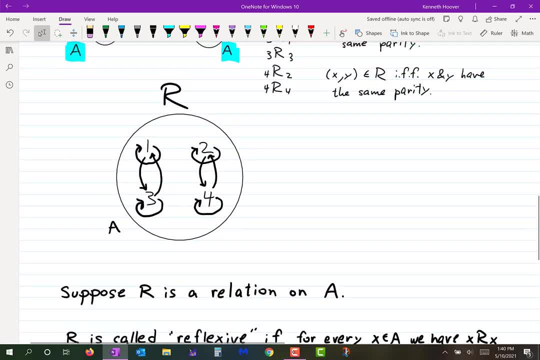 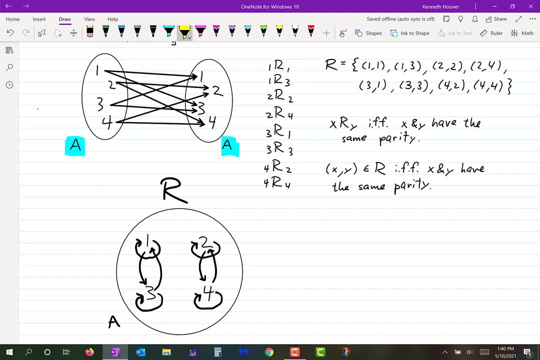 example, here is this one reflexive. let's um, let's look here. the easiest way to tell is probably here. let's look at that, okay, and I want you to notice a few things here. notice that 1- 1 is in the relation, 2, 2 the relation, 3, 3 is in the relation and 4- 4 is in the. 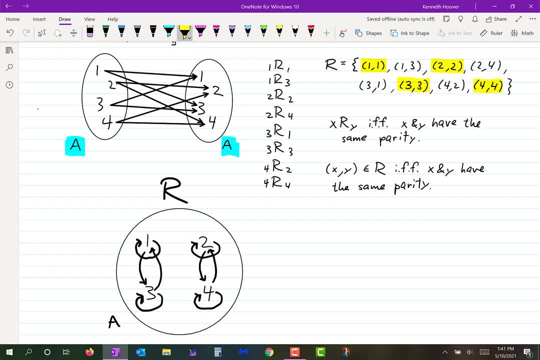 relation. what's that tell you? tells you: the relation is reflexive. every number in a is a reflexive, is related to itself in the relation are: ok, let's see if this one is symmetric. this takes longer. so let me ask you this. let's do this. so here's 1. 1. let me ask: 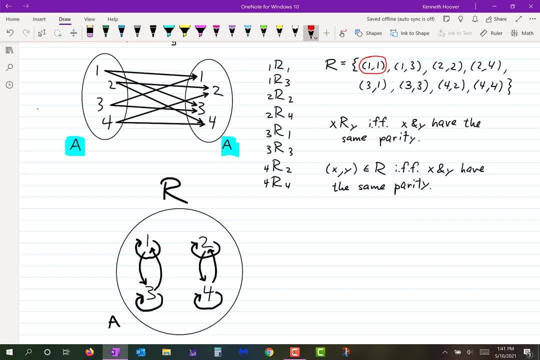 you this question. I'm going to flip that order and instead of 1, 1 is going to become 1, 1. Okay, Is 1, 1 in there? Yes, it is Now. that one wasn't interesting because the first number and the second number are the same, But it becomes more interesting here. Here's 1, 3.. I'm going to flip that order and get 3, 1.. Can you find 3, 1 in the relation? Yes, Right there, Okay. 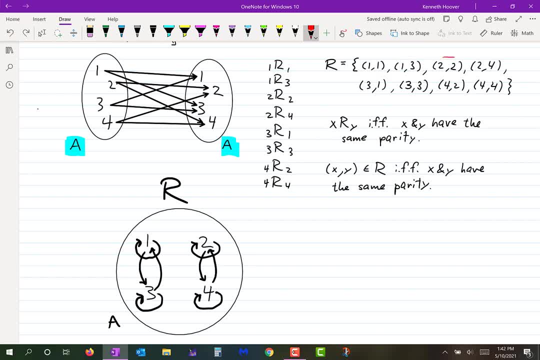 Here's 2, 2.. Is 2, 2 also there? Yes, it is Here's 2, 4.. Is 4, 2 also there? Yes, it is Here's 3, 1.. Is 1, 3 also there? Yes, it is. 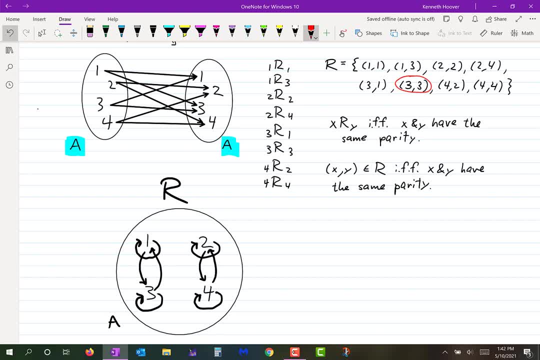 Here's 3, 3.. Is 3, 3 also there? Yes, it is. Here's 4, 2.. Is 2, 4 also there? Yes, it is. And here's 4, 4.. Is 4, 4 also there? 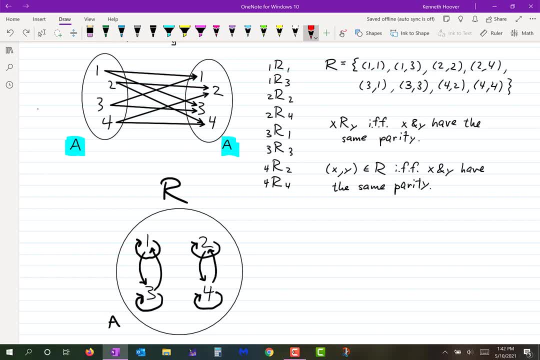 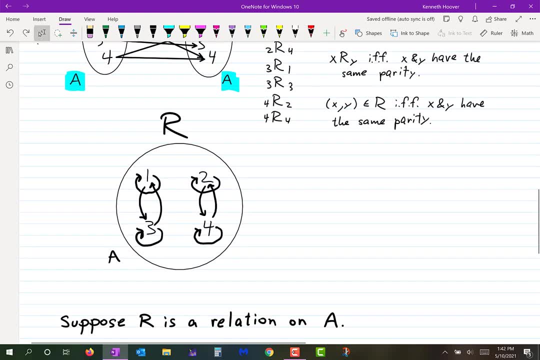 Yes, it is So. that relation is symmetric, So it is reflexive and it is symmetric, Okay. Another way to do that is to look here for reflexivity. You look to see if every number is related to itself, And it is, So that means it's reflexive. 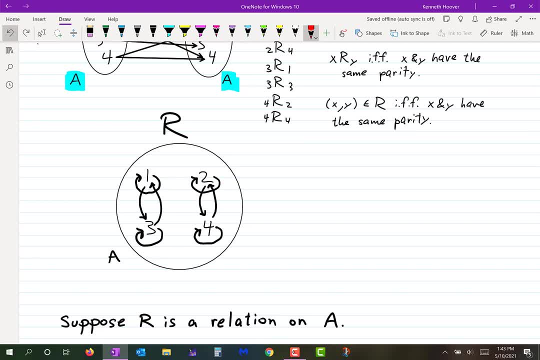 For symmetry, you have to see if every arrow can be reversed, And they can. Every arrow can be reversed, So it is symmetric. Okay, So having the same parity is reflexive and symmetric, At least on this particular set. 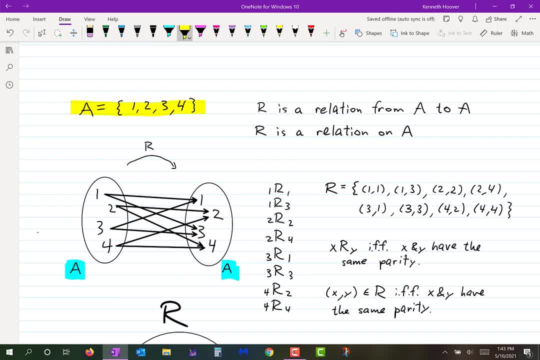 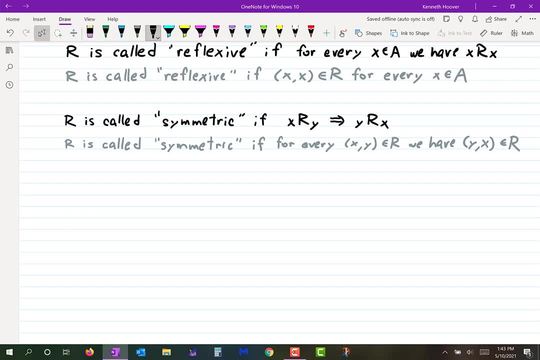 But even if that set was all real numbers, it would still be reflexive and symmetric. Okay, Now one more adjective called transitivity. Okay, R is called transitive If X being related to Y. 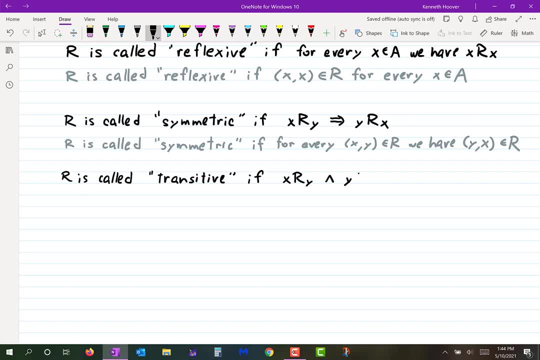 and Y being related to Z together imply that X must be related to Z. Another way of saying that R is called transitive if xy being an element of r and yz being an element of r imply that xz is an element of r. 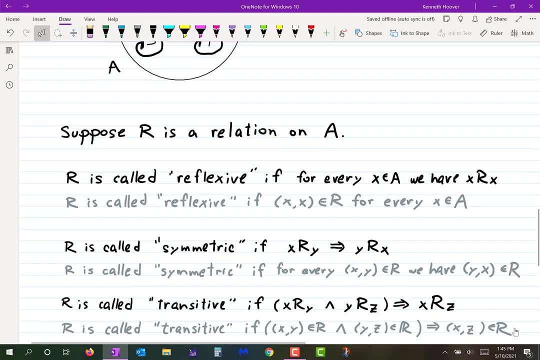 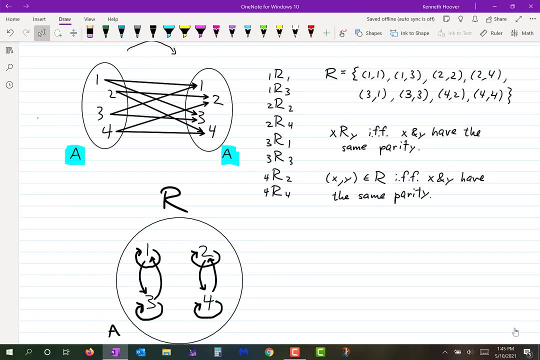 let's look at our second example. we saw that it is reflexive and symmetric. is it transitive? this one takes a long time to check because if you check it manually, there's so many things to check- let me think for a second of how many it would. 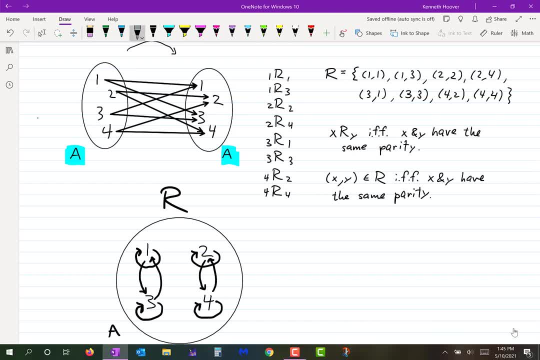 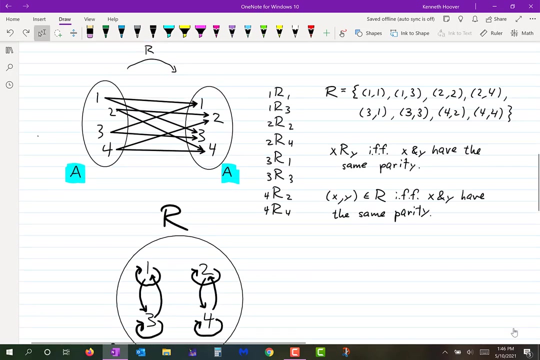 there's eight elements of our relation. to see if this is reflexive, I would have to check 64 possibilities. I'm not going to check all 64 with you, but I'll point out some of them. whoops. here are the types of things you would have to check. 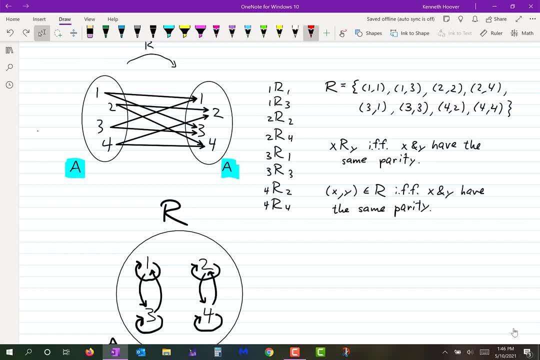 for transitivity, you would have to say, for instance, 1,3 is in there and 3,3 is also in there, so 1 is related to 3 and 3 is related to 1. does that imply that 1 is related to 1?? 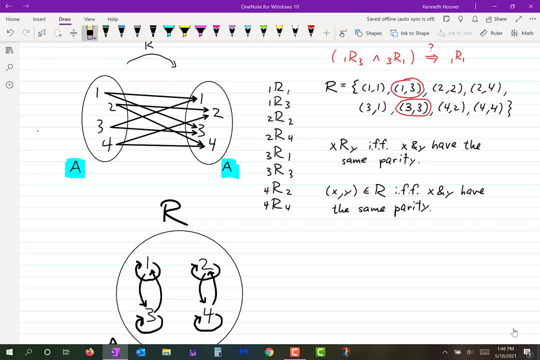 and the answer is yes, because 1,1 is there as well. ok, those are the type of things you'd have to check. here's another one just as an example. I could say: 2 is related to 1, 2 is related to 2. 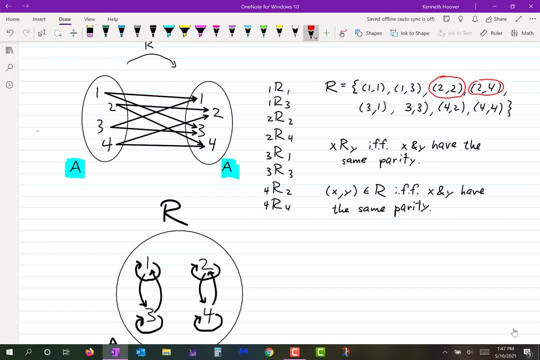 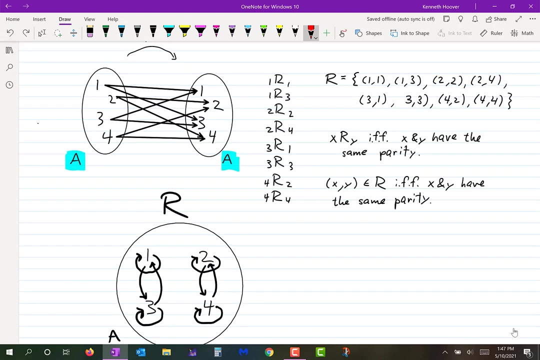 and 2 is related to 4. is 2 meaning this here, related to 4 meaning this here? and the answer is yes, because that's right here. ok, you see how that works. if you're looking at the diagram with arrows, then this is how it looks. 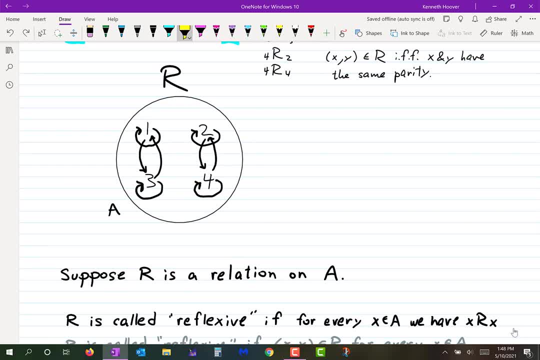 you would ask yourself: if I follow one arrow, let's say from here to here, let me choose a different example. if I follow one arrow, let's say from 1 to 3, and then from there I can follow another arrow, from 3 to 1, 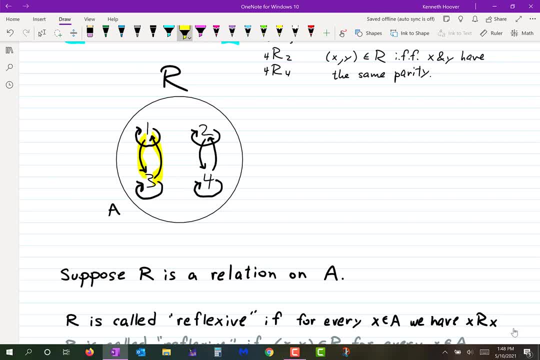 could I have gotten from the beginning to the end with only one arrow instead of needing two? and the answer here is, in this case, yes, I could have just gone on this arrow here, you see. so that's an example of transitivity, but the relation is only transitive. 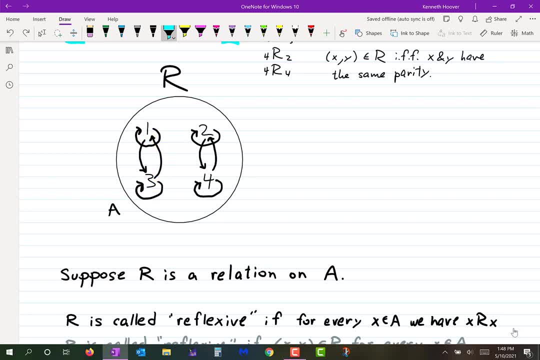 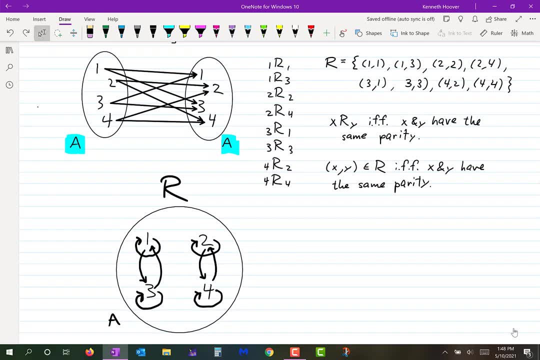 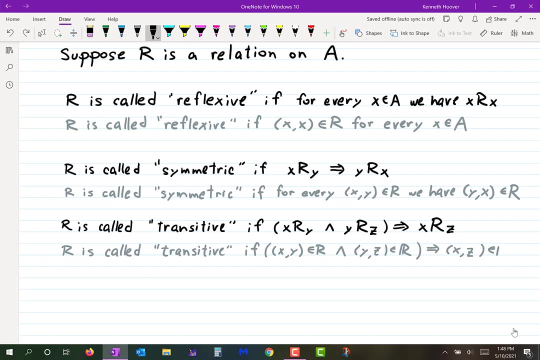 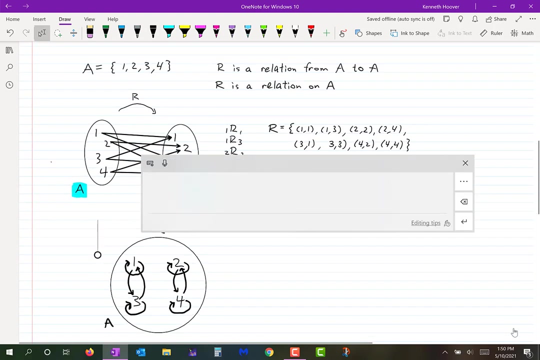 if all such possibilities exist. so transitivity takes a long time to check. ok, now here's another word. r is called an equivalence relation if it is reflexive, symmetric and transitive. ok, ok, let's look back at our example. is this relation the relation of having the same parity? 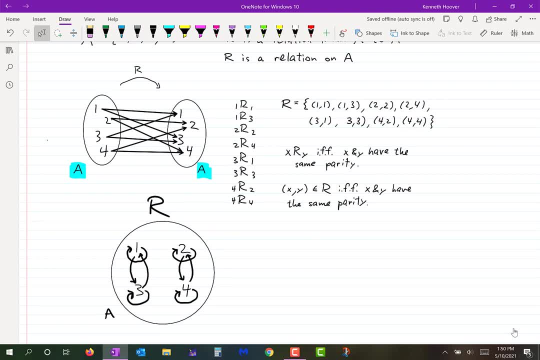 is that an equivalence relation? then? the answer is yes, because we checked it and we saw it's reflexive. it is symmetric and, even though we didn't check transitivity thoroughly, I think I think by looking at it for a few minutes you will see that it is in fact transitive. 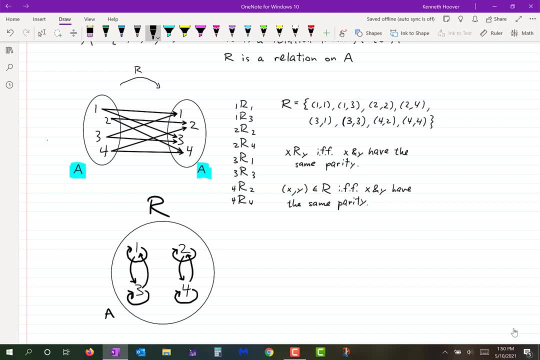 so having the same parity is what's called an equivalence relation. ok, and what that means? the reason why we call it an equivalence relation is this: you're probably used to equivalent meaning equal to, and so you might think: well, that's weird to call this an equivalence relation. 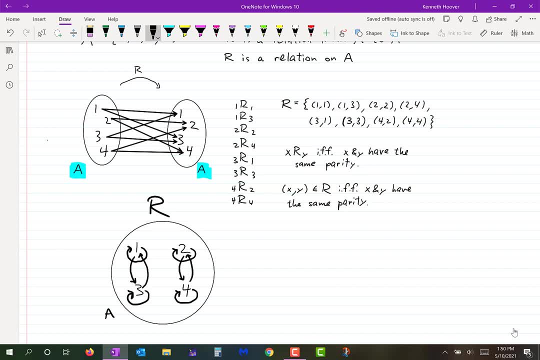 because we said that 2 is related to 4, but certainly they're not equal. but there is a reason why we call it an equivalence relation, and that is this: if the only thing that you care about is parity and nothing else, so oddness and evenness. 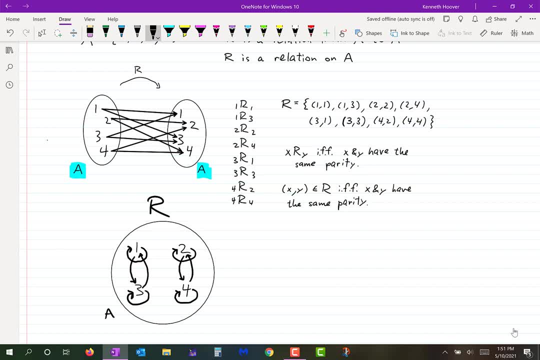 if that's the only thing you care about and nothing else, then as far as you care, 2 and 4 are the same number. ok, you gotta. don't ignore the first half of that sentence, though, because that's the important part. if the only thing you care about. 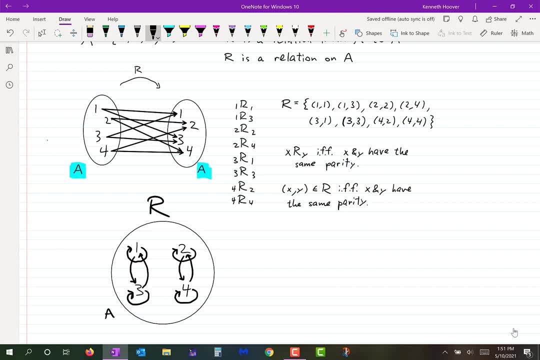 is parity. ok, let's talk about this for a minute. I'm not going to write anything out, so you have to listen very carefully. ok, I'm going to play devil's advocate on that, so I'm going to say it again: having the same parity is reflexive. 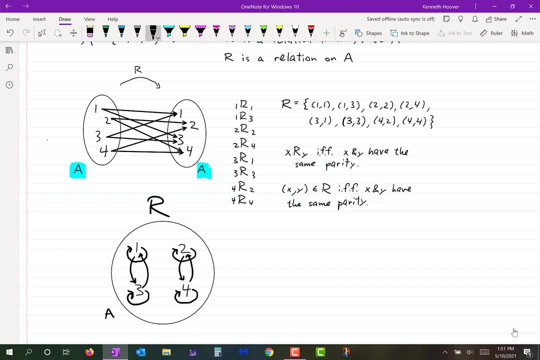 symmetric and transitive, so it's an equivalence relation. that means if the only thing you care about is parity, then 2 and 4, as far as you care, are the same number. now you might say: well, that can't possibly be true because, for instance, 2 times 3 is 6. 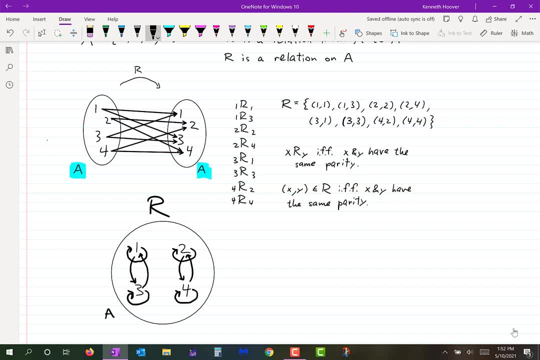 and 4 times 3 is 12. so if 2 and 4 are the same number, as far as I'm concerned, then that means 6 and 12 would have to be the same number, and my answer to that question is: yeah, you're right. 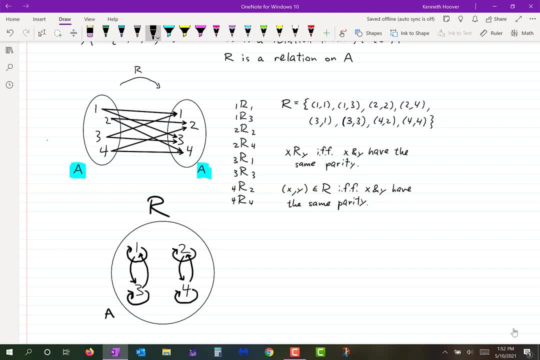 if the only thing you care about is parity, then 6 and 12 would be the same number. because why? because they have the same parity. see what I'm saying. alright, now one more concept to cover if you have an equivalence relation. oh, by the way, sorry. 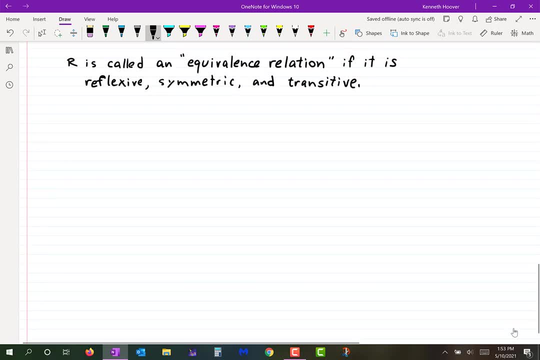 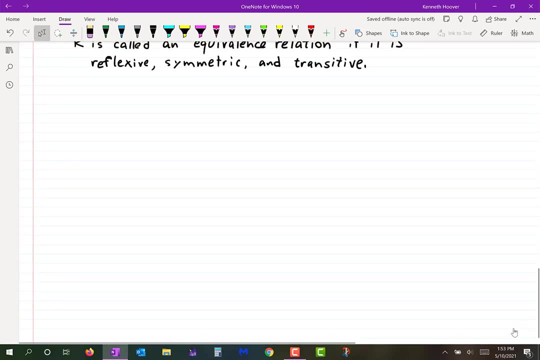 let's. let's look at a new example for a minute. same set, ok, the set of numbers 1, 2, 3 and 4. same set, but this time I'm going to do a different relation. ok, 1, 2, 3, 4, I'm going to do. the relation is less than. 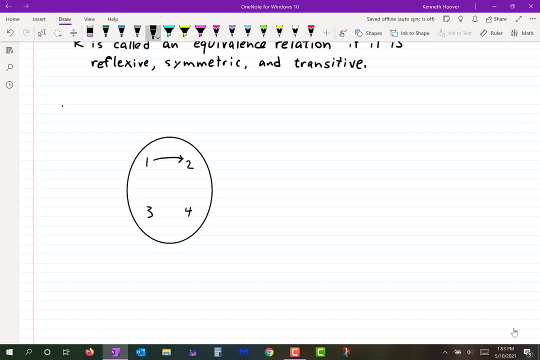 so it's true that 1 is less than 2, 1 is less than 3 and 1 is less than 4. 2 is less than 3 and 2 is less than 4. 3 is less than 4, and that's it. 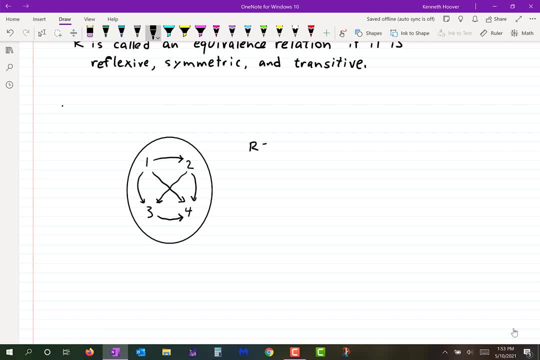 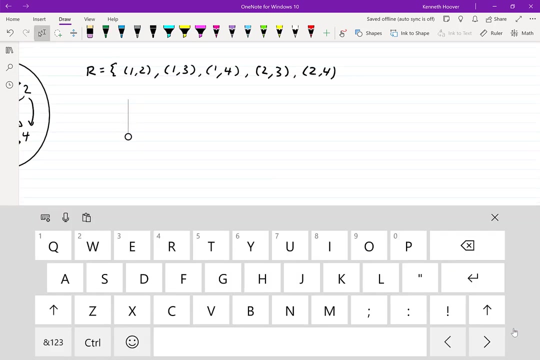 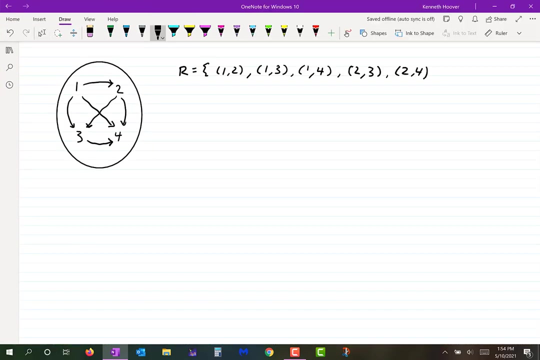 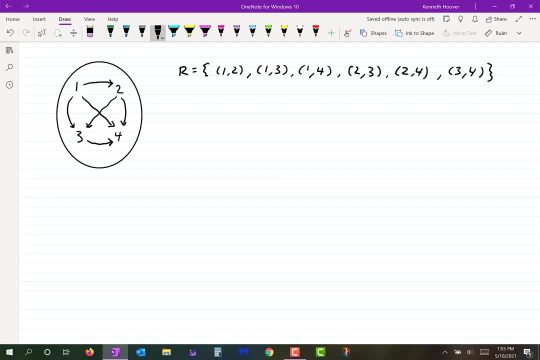 than 2.. 3 is not less than 3.. 4 is not less than 4.. It's also not symmetric: 1 is less than 2, but 2 is not less than 1, and so on and so on. It is, however, transitive If. 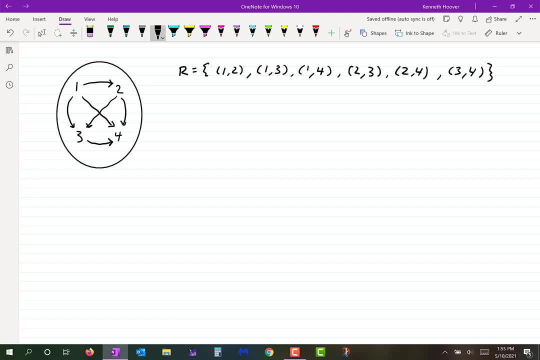 one number is less than a second number and that second number is less than a third number, then the first number is going to be less than the third number. So it is transitive, But it's not reflexive or symmetric and therefore it's not an equivalence relation. Okay That. 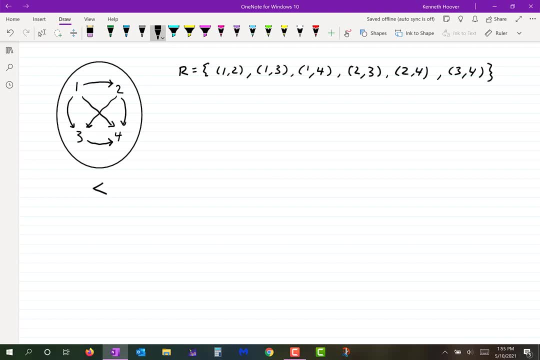 is the relation less than. I could make it reflexive by changing it to less than or equal to, and then that would add less than or equal to, less than or equal to less than or equal onto, and so on and so forth. O, m, e, a, t, q, r, x, e and so forth. So I could 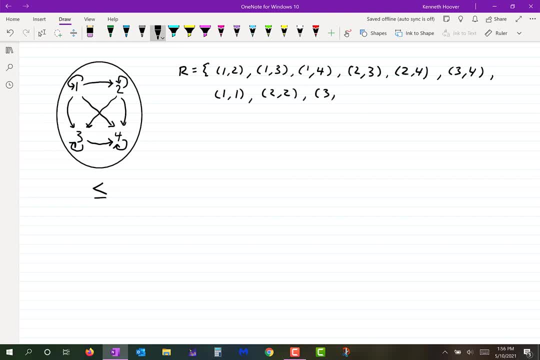 epsilon equal to B and I would have equal to b as well. So I수� feedback would be A and E would be b. Okay, Okay, blond and blue and green and orange and blue and blue and green and green and red and. 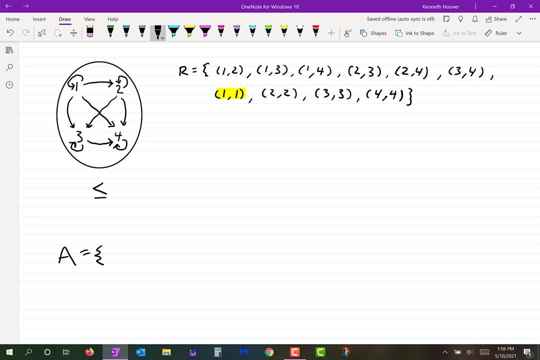 started out with a set- 1, 2, 3 & 4- and we see that every element of a is related to itself by the relation less than or equal to, so it is reflexive. the relation less than or equal to is reflexive on a. it is also transitive, but it's still not. 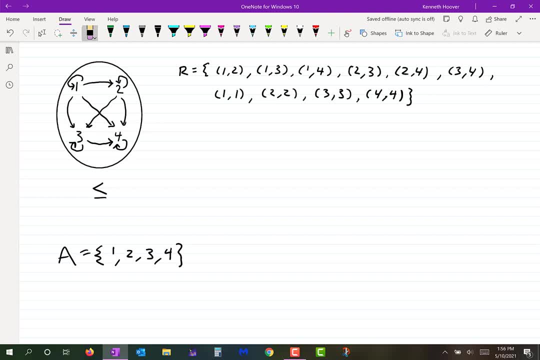 symmetric, for instance ones related to 2, but notice that 2 is not related to 1. what else could I say for about? three is related to four, but four is not related to three. okay, so it's still not symmetric, it's reflexive and transit, but 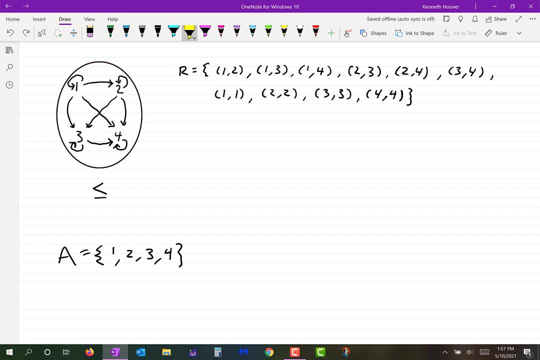 not symmetry. so this is not an equivalence relation. okay. once again, why do we use the word equivalence if all I care about is less than or equal to? so let's say order. if all they care about is order, okay, then I can say that the numbers one. 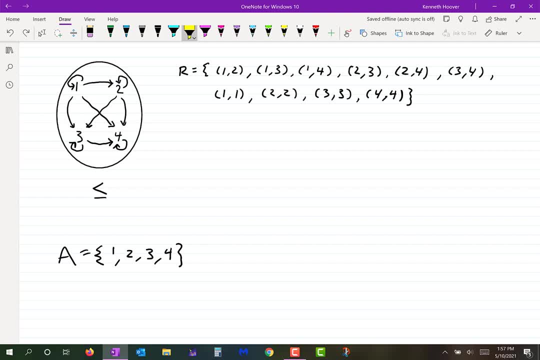 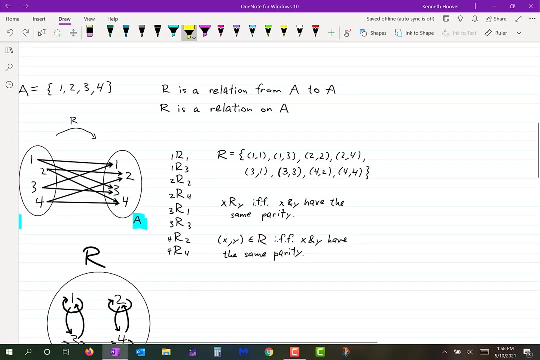 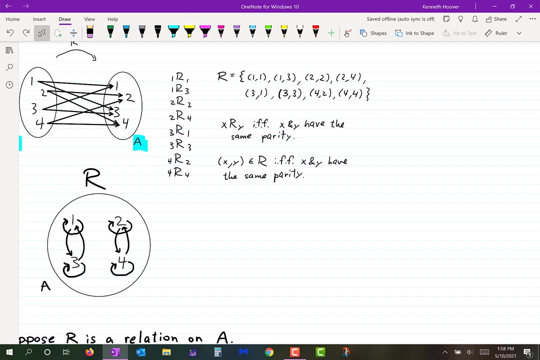 and three are not the same in my mind, because one comes before three but three doesn't come before one. so if I'm if I care about order, then in my mind one and three have to be kept separate. they are distinct concepts. whereas, going back up here, if what I care about is parity being even or odd, then as far as I care, 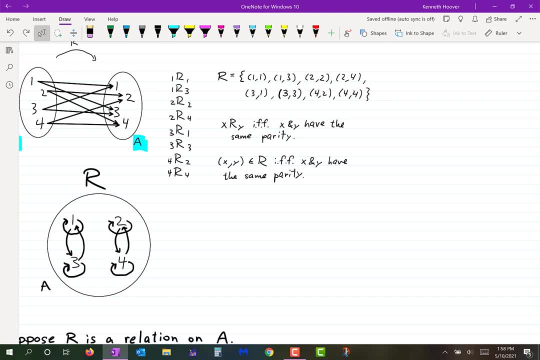 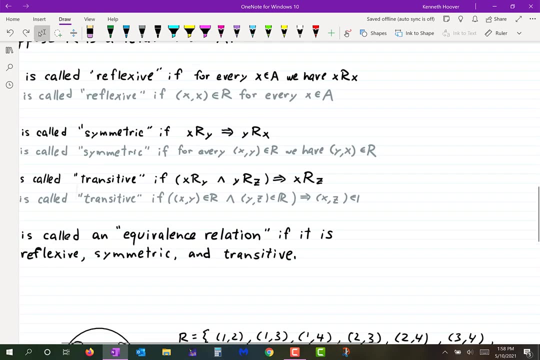 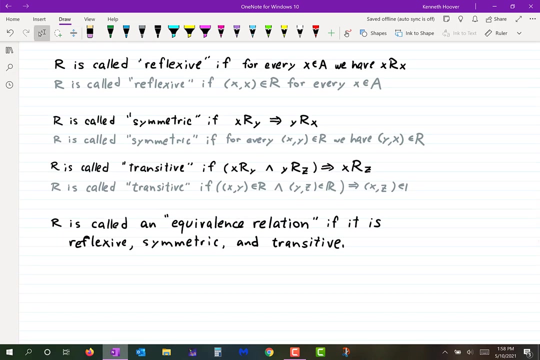 one and three are the same. they represent the exact same thing. okay, they represent the same concept, which, in this case, would be oddness. okay, now there's something that I wanted to say before and I said: let's wait a minute and and look at something that's. 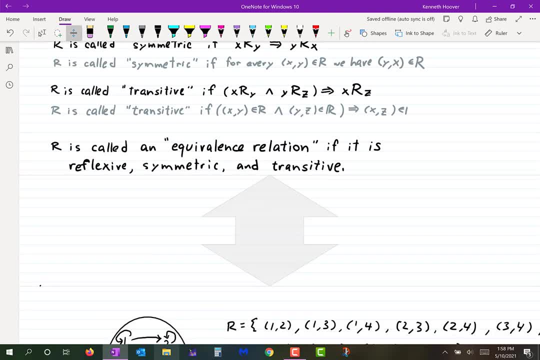 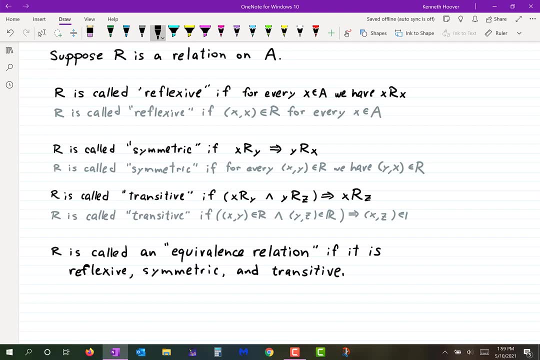 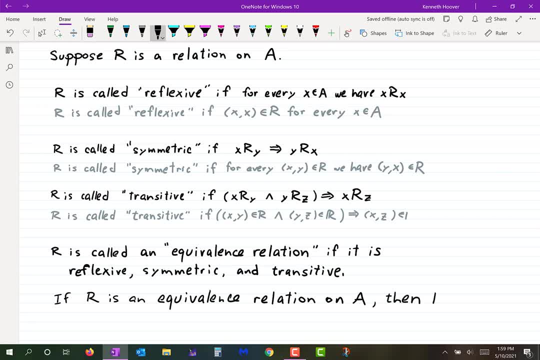 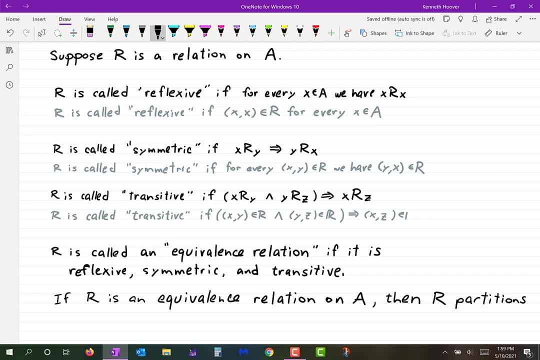 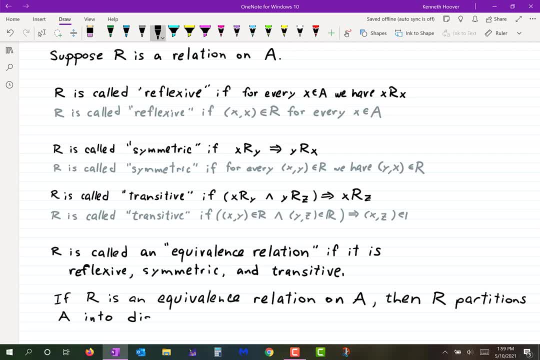 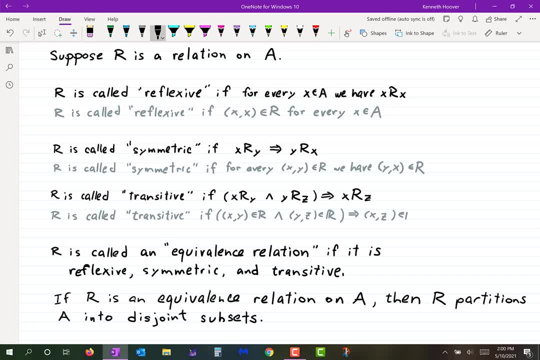 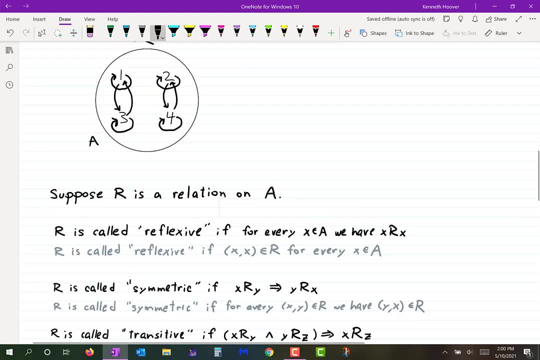 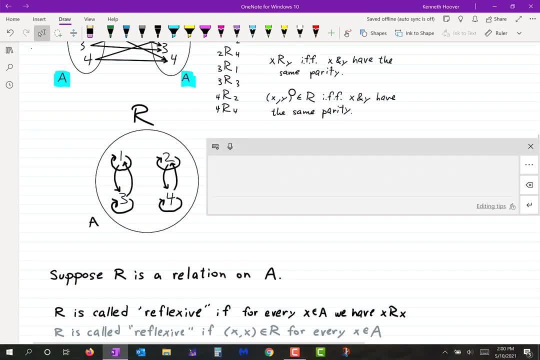 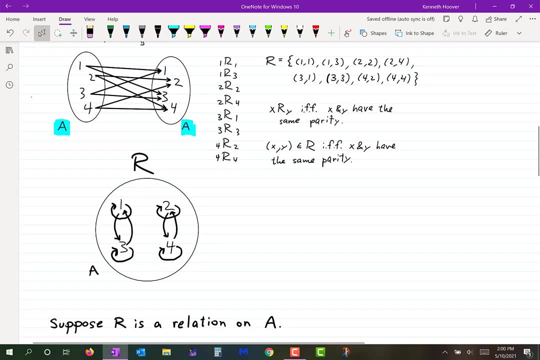 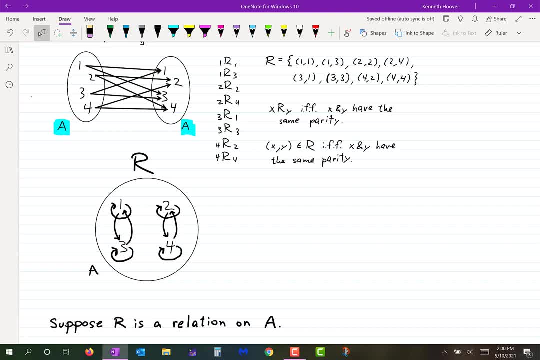 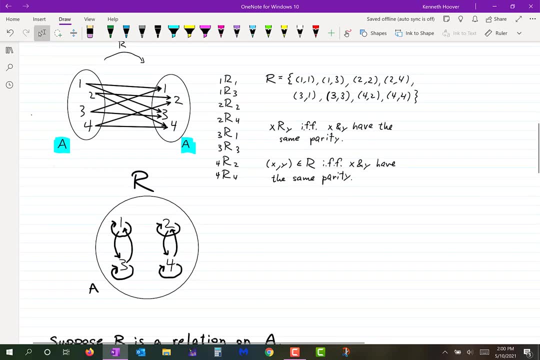 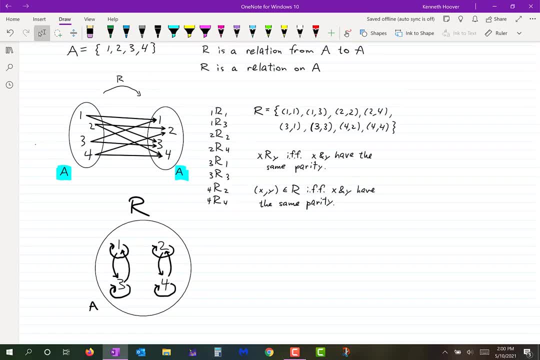 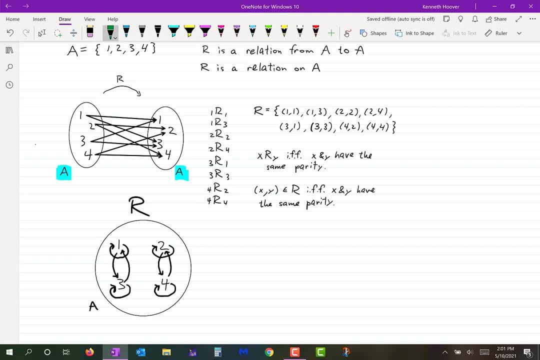 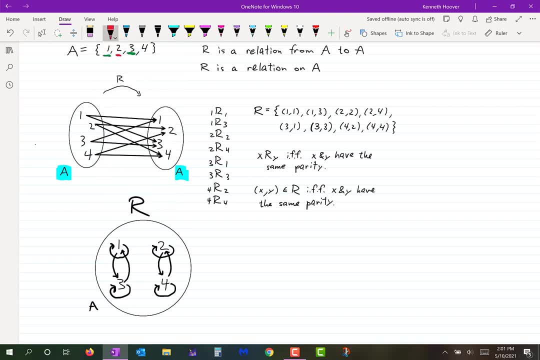 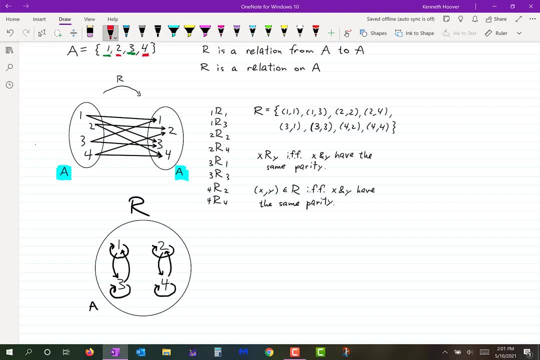 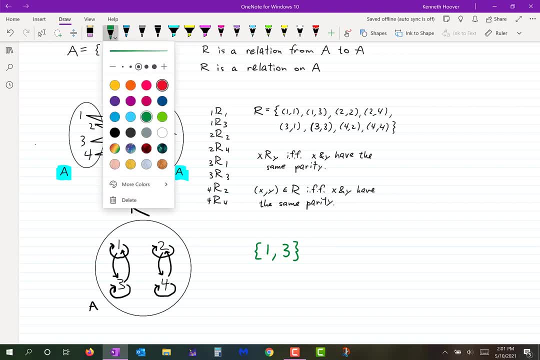 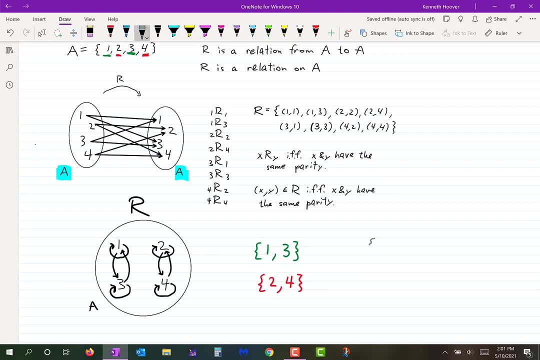 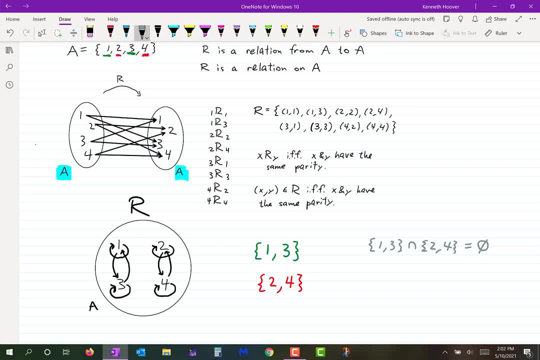 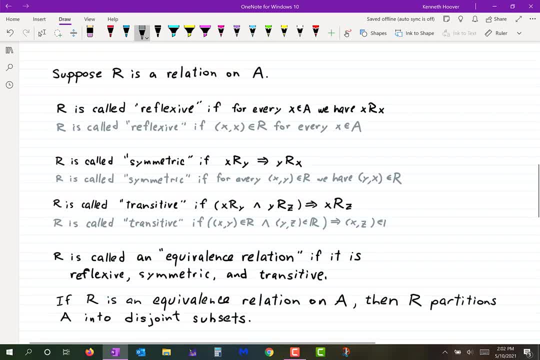 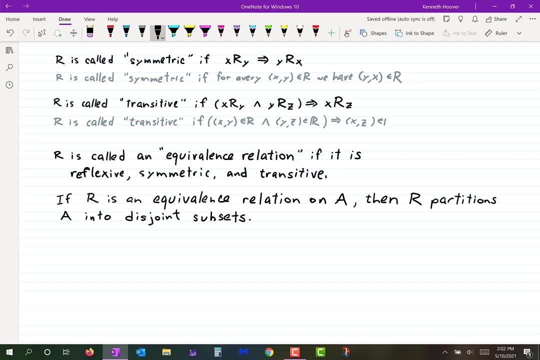 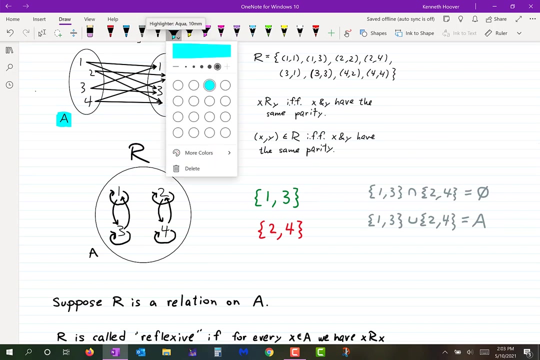 equivalence classes. so let's go back to where we're writing definition. if R is an equivalence relation on A, then R partitions A into disjoint subsets. let's change that period to a comma and let's say called equivalence classes. okay, so going back up here, that green set right here. of course I wouldn't say 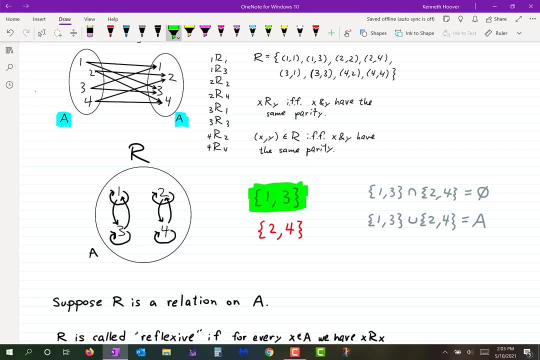 that's the green equivalence class, because maybe somebody else doesn't have colored pencils and they didn't use green. you would say that is the equivalence class of one, or you could call it the equivalence class of three. The equivalence class of 1 and the equivalence class of 3 are the same equivalence class. 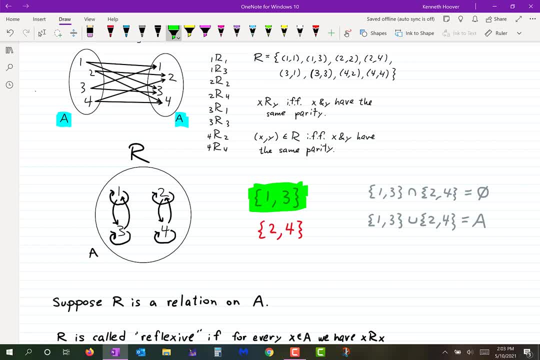 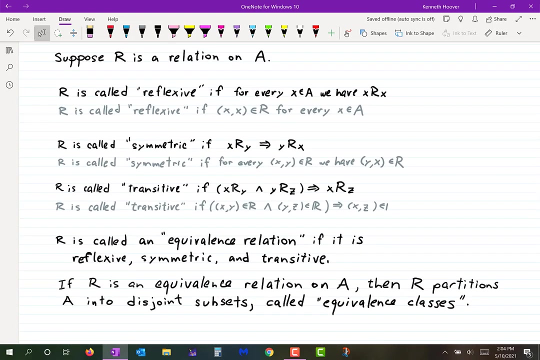 They are the set consisting of 1 and 3.. The other one, you can say that's the equivalence class of 2, or it's the equivalence class of 4.. Okay, And, by the way, an equivalence relation oftentimes gets this symbol, an equal symbol, except with 3 bars instead of 2.. 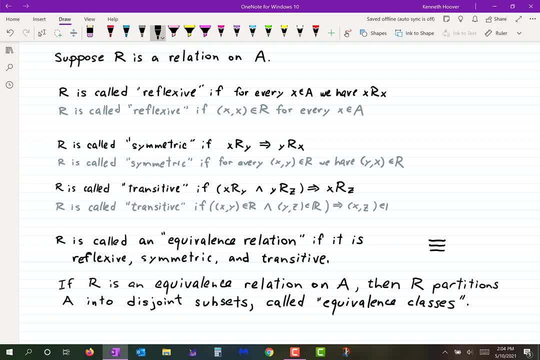 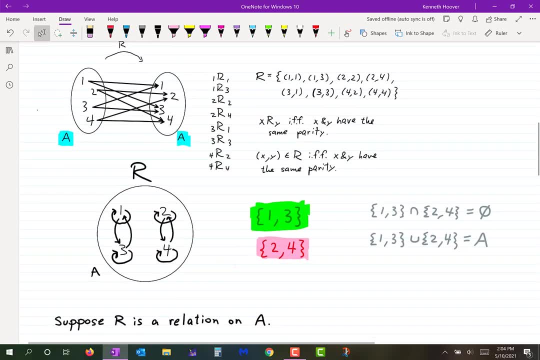 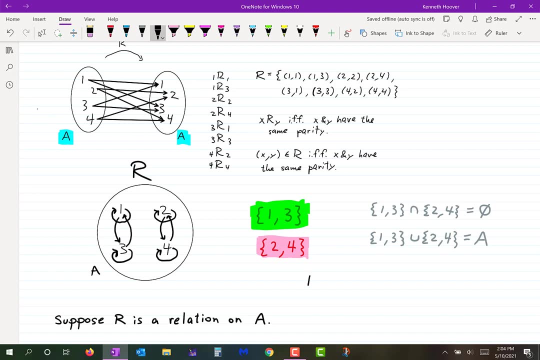 That is often used for equivalence relation. Anytime you see that it means you have an equivalence relation. So up here I can say, and it would be correct to say: 1 is equivalent to 3.. 4 is equivalent to 2.. 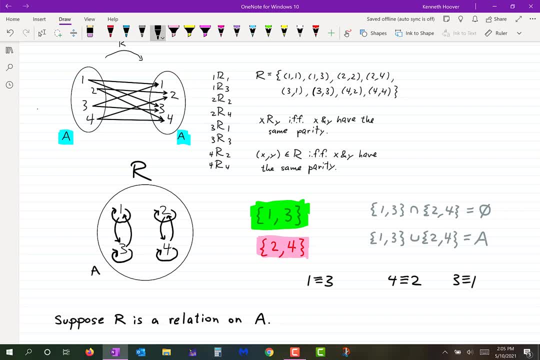 3 is equivalent to 1.. It's unnecessary to say 3 is equivalent to 1, because I know equivalence relations are symmetric. So when I said 1 is equivalent to 3, I was automatically. I was automatically saying also 3 is equivalent to 1, so it's not necessary to say that separately, okay. 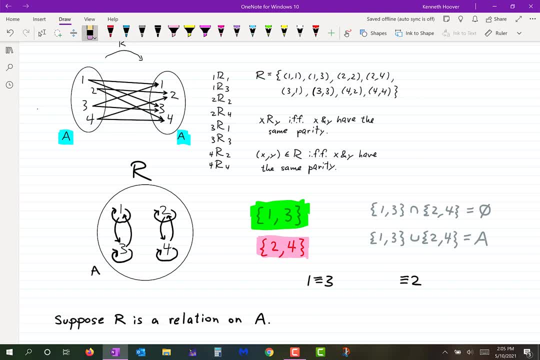 And I said 4 is equivalent to 2, but I could have just as easily said that 2 is equivalent to 4,. okay, Now the only drawback to this symbol right here: that's just a generic symbol for equivalence relation. 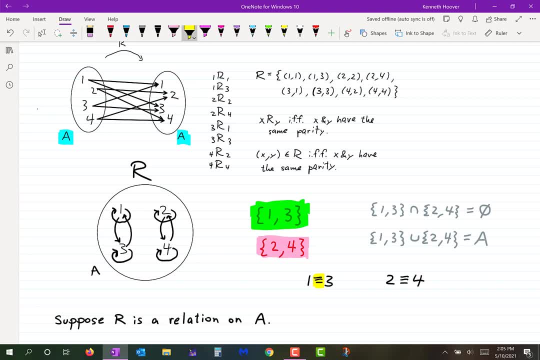 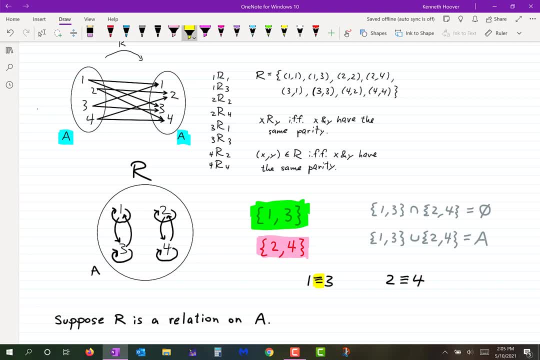 If I wrote that you have no way to know what the relation is, You have no way of knowing that that relation is having the same parity, For all you knew that relation might have been. Well, I don't want to just make up something off the cuff, okay.